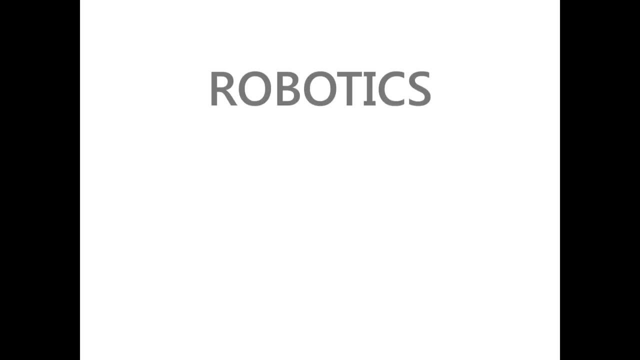 Okay, so let's move into our topic Today. I will provide a brief overview of the robotics industry, then move into a discussion of current robot safety regulations and standards. These standards are complex and rapidly changing, so our goal is to ensure that webinar attendees leave today knowing what standards are current, what has recently been updated and what changes are in the works. 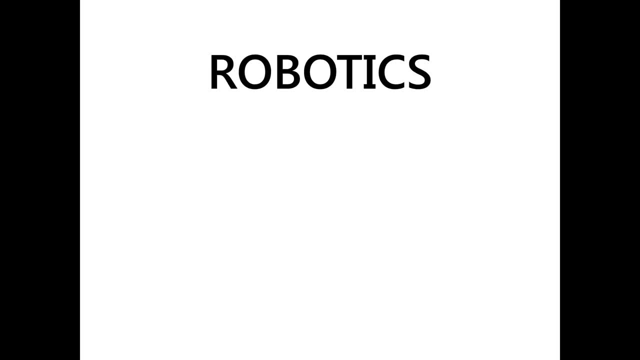 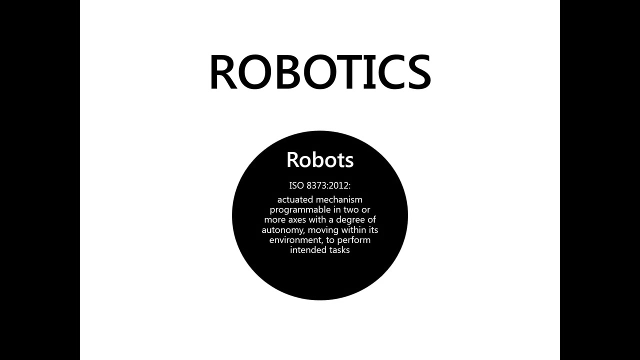 Then I will turn the presentation over to Roger Roger, who will provide a more detailed review of different robot safeguarding techniques and application examples. Today's presentation is only a robot safeguarding primer and designed for a non-technical audience, So let's define what we are talking about. As defined by ISO 8373-2012,, a robot is an actuated mechanism programmable in two or more axes. 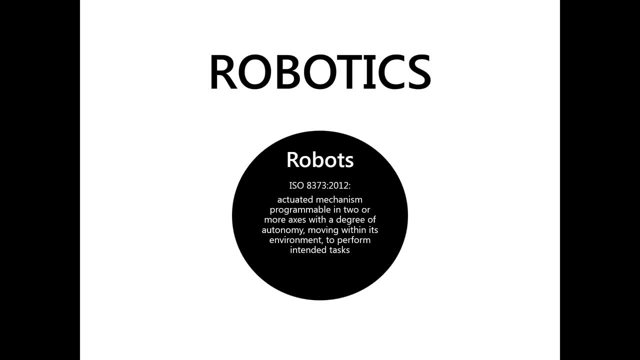 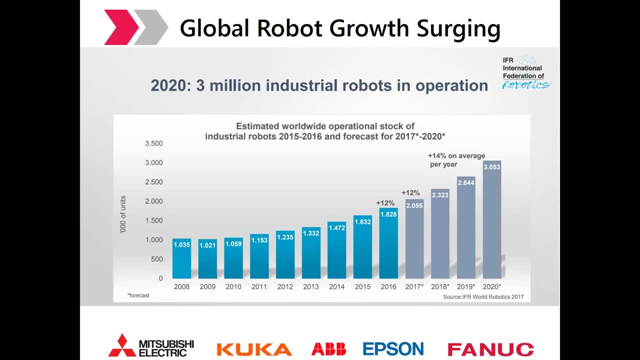 with a degree of autonomy moving within its environment to perform intended tasks. Today, there are over 2 million robots deployed in global factories And that number is expected to exceed 3 million by 2020, representing a 14% compound annual growth rate, or CAGR. 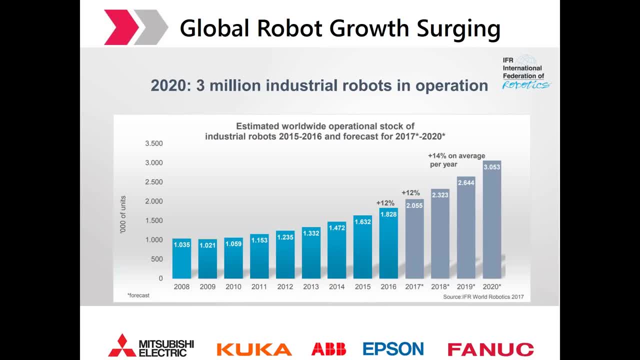 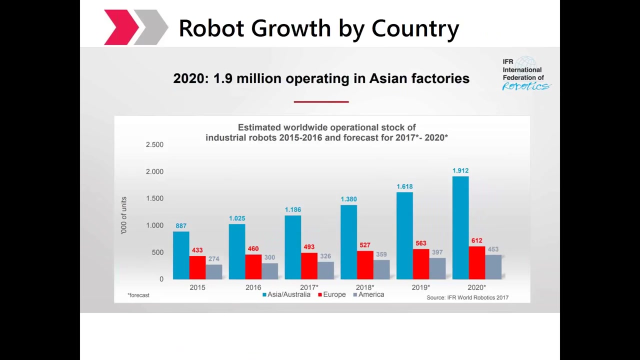 between 2018 and 2020, broken down by sectors. around 70% of industrial robots are currently working in automotive, electrical electronics, metal and machinery industry segments. The vast majority of robots live in Asia, followed by Europe and America. 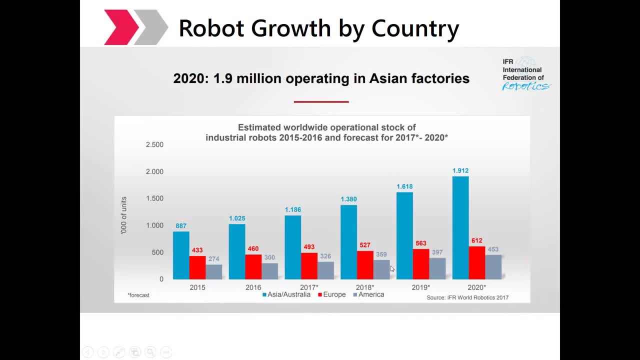 Today, there are approximately 350,000 robots operating in American factories, with robot density at 189 robots That's, per 10,000 employees. The main driver of this growth is the ongoing trend to modernize factories and automate production in order to strengthen American industries. 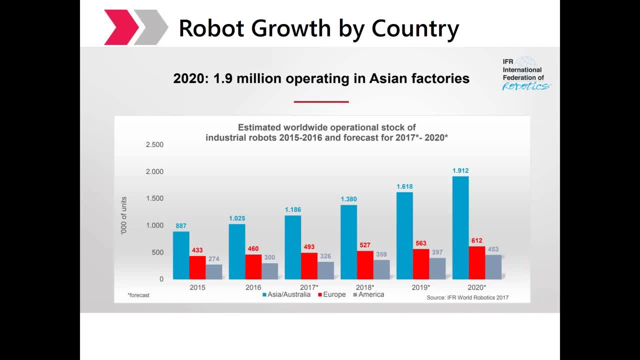 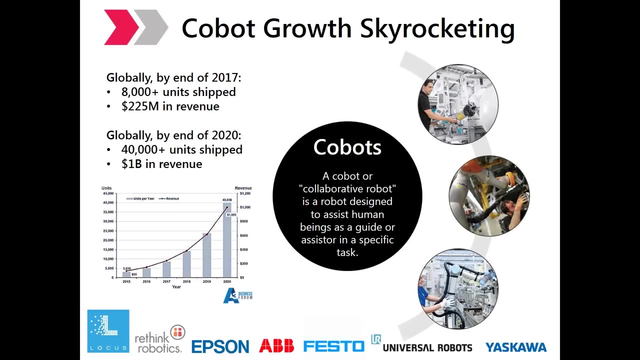 in the global market and to keep manufacturing at home and, in some cases, to bring back manufacturing that had previously been sent overseas. So long story short: robots are here to stay. So what is a collaborative robot, or cobot for short? 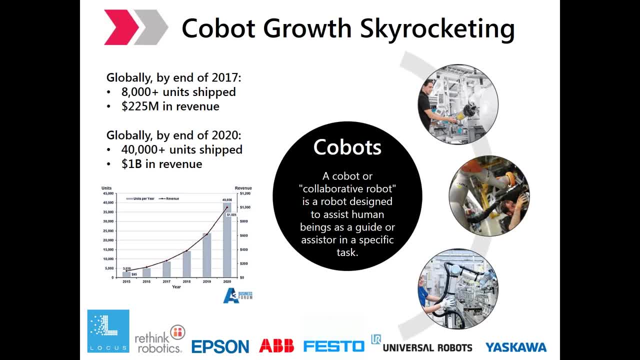 Well, There is no global industry standard definition yet, but it is generally considered to be a robot designed to assist human beings as a guide or a sister in a specific task. Cobots have been around since the 1990s, But in recent years, advancement in sensors and automation 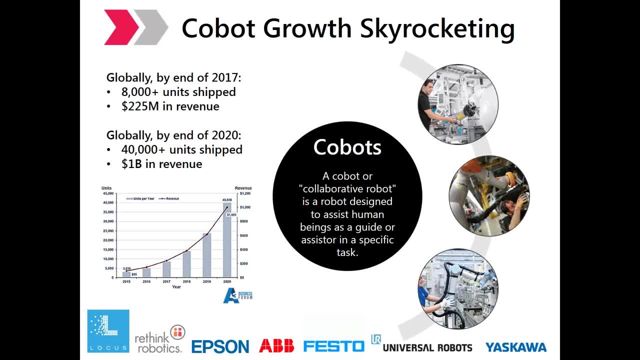 technology, not to mention artificial intelligence or AI, have raised their profile quite substantially. A regular industrial robot is designed to be programmed to work more or less autonomously. Robots in industry have always been big, strong, robust devices that work on specific tasks designed for them. 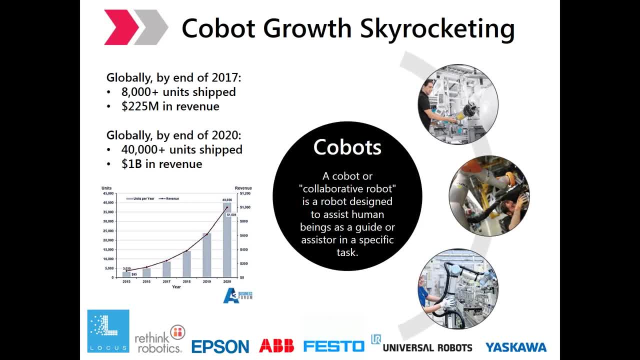 They're surrounded by fences and guards for safety purposes. Their bright colors are used to warn the surrounding workers about the danger they represented, And a lot of programming skills were necessary to bring up these industrial robots- Cobots, in fact, are the opposite. 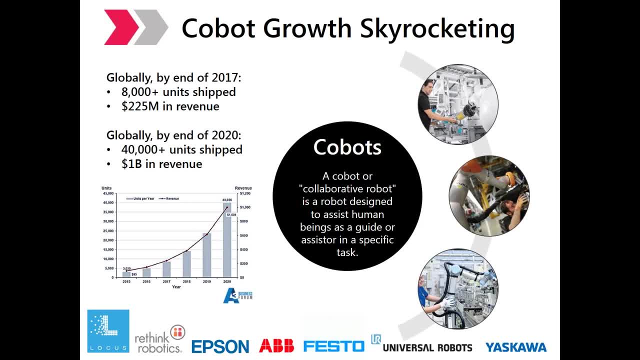 They are compact, lightweight And have integrated sensors, passive compliance or overcurrent detection, and safety features. The integrated sensors will feel external forces And if this force is too high, the robot will stop its movement. The cobot space is growing rapidly. 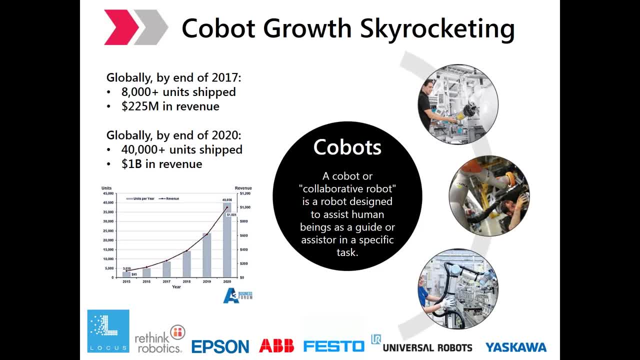 But it is only one tenth of the size of the installed industrial robot space today. Experts predict that the cobot market will be worth over a billion dollars and some analysts predict $3.3 billion by 2020, driven primarily by adoption in the automotive, metal and machining, furniture and equipment, food and beverage. 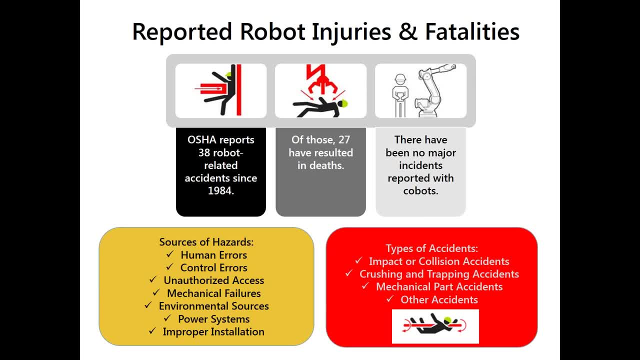 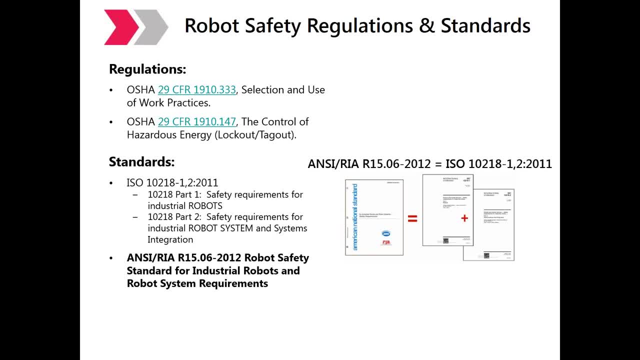 that were physically moved or installations that have changed after 1999 should undergo review that they remain compliant and, as always, a risk assessment is the best option for that review. and a new standard is in development called ANSI RAA R 15.08, which deals with industrial mobile robot. 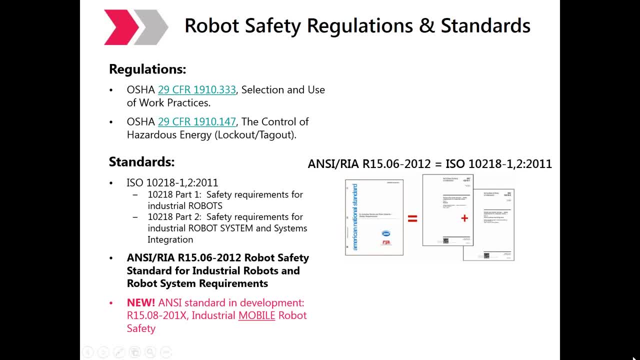 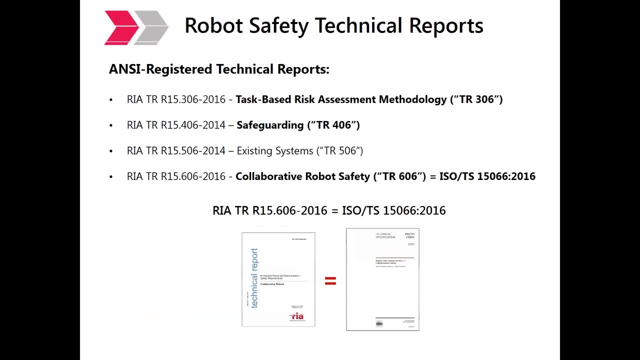 safety. so the key word here being mobile mobile bases. this standard is expected to debut sometime before 2020. so there you have it. okay. there are also several ANSI registered technical reports, or TRs, which are supplemental to ANSI RAA R 15.06 2012 and are intended to be applied in. 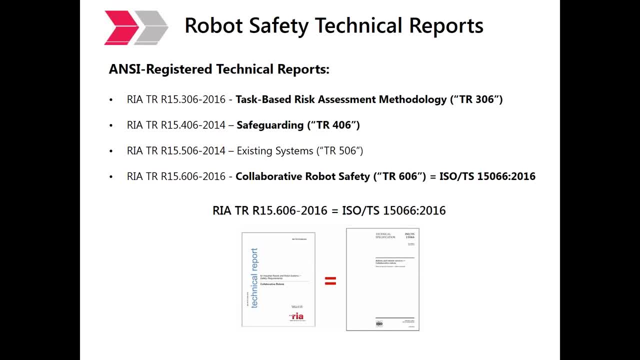 conjunction with the requirements outlined in the standard. the information contained in the technical reports is informative, meaning written with words like should, whereas the standard itself is normative and written with words like shall. so just to go through these quickly: TR REE 6 is OOOOOOO. 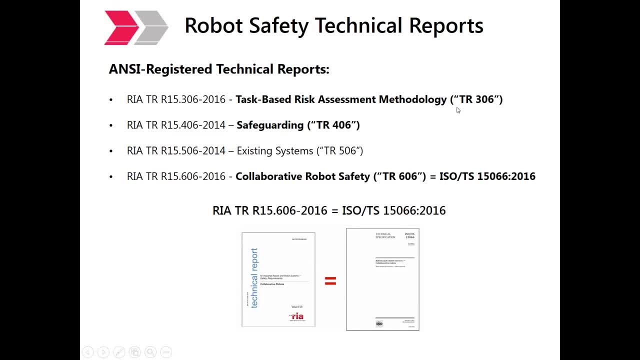 is the technical report that is all about task-based risk assessments. Technical report 406 is all about robot safeguarding, Technical report 506, existing systems And technical report 606,, which was just issued in 2016,, is all about collaborative robot safety. 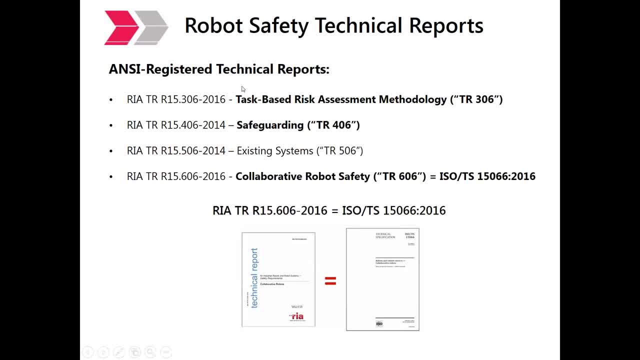 Please note that the task-based technical report 306 was revised in 2016,, so make sure that you're on the current version of these technical reports. So the TR-606, which was issued again in 2016,, is actually the same thing as ISO TS-15066-2016.. 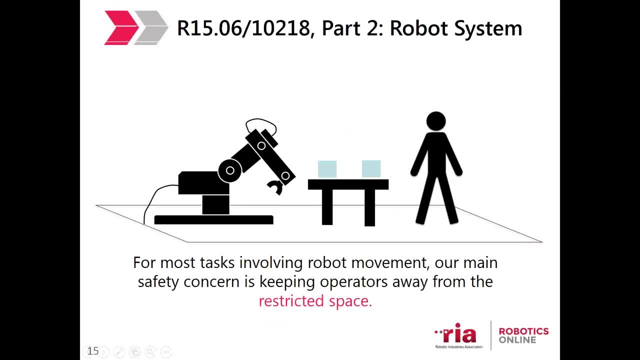 So those are interchangeable as well. The first version of R-1506 was written in the 80s, And at that time the traditional robot approach was that the robot is fixed, mounted in place and doing something that could potentially be dangerous to humans, such as welding or painting. 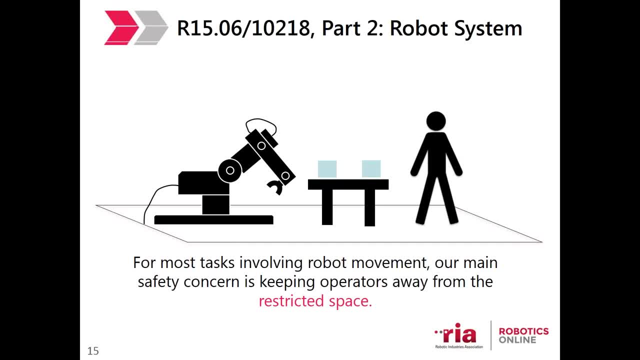 So most tasks involving robot movement. based upon these assumptions, our main safety concern is keeping operators away from the restricted space or the swept volume of where the robot fully extended robot arm could potentially reach while in operation. So to keep the humans safe, we kept them out of that area. 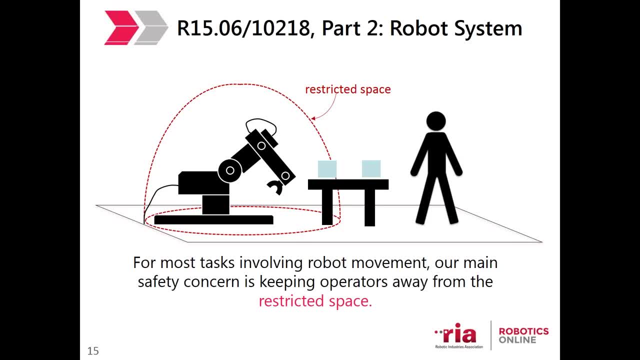 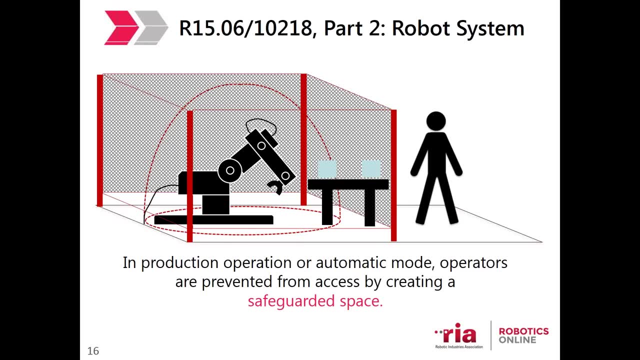 And the easiest way to do that is to create a safeguarded space. So in this example we see a perimeter guard installed on all four sides of the work cell, which again is a designed to keep the human out of the safeguarded space. 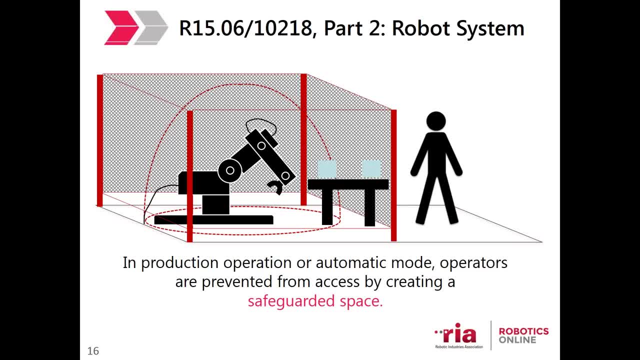 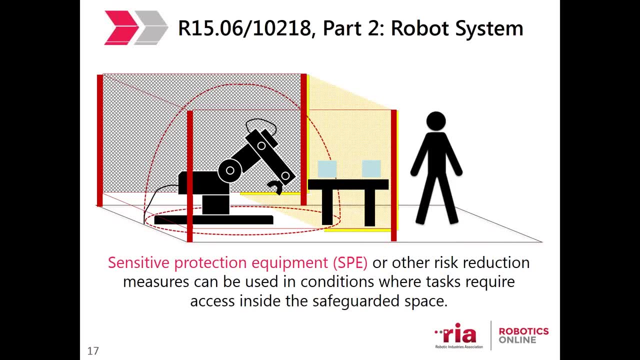 Now there are going to be some times when the human needs to enter the safeguarded space, such as to perform maintenance, testing, clear jam, et cetera. In those situations, we can safeguard the work cell using sensitive protection equipment or SPE. 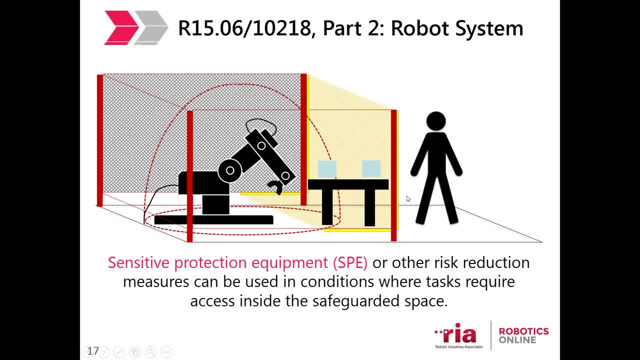 such as pressure-sensitive mats and light curtains. Once the human trips the safeguarding, either by breaking the light curtain beam or stepping on a safety mat, the safeguarding equipment will turn off the robot so the human can enter the area safely. This is just one example of potential SPE equipment. 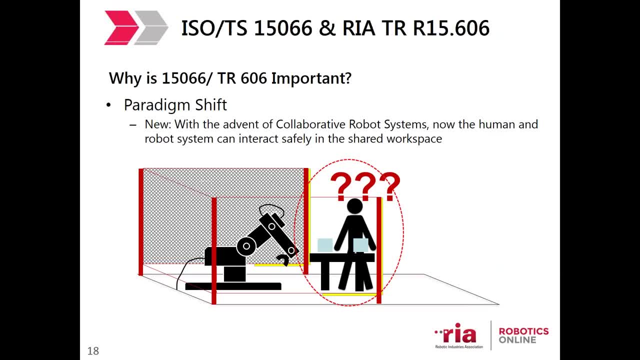 that can achieve this goal. But what happens when the human and the robot need to interact? In R-1506,, the standard permits both collaborative and mobile robot systems, But does not go into great detail about how to achieve these safely. That's why TR-606 is so important. 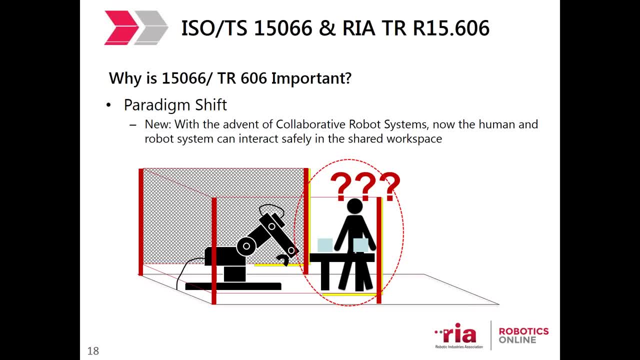 because it represents a paradigm shift whereby the human and the robot system can interact together in a shared workspace. because collaborative robot systems will have built-in safety capabilities that reduce risks to the human worker. So why is TR-606 so important? Well, basically, a lot of this information. 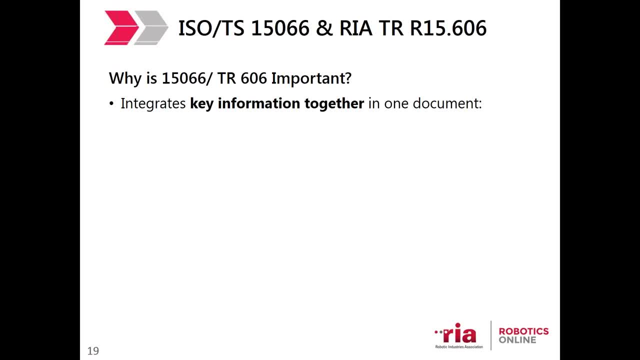 was included in a variety of documents, And TR-606 really pulls it all together in one handy document and includes definition of collaborative robot operation, safety-related control systems, factors for the design of the collaborative robot system, built-in safety-related systems and then, of course, the robot system. 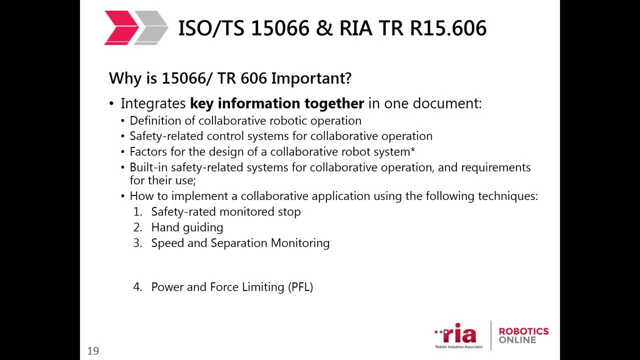 And TR-606 also includes information on safety-related systems for collaborative operation and requirements for their use, including how to implement a collaborative application using the following techniques. So these four- here are actually four different types of cobots: safety-rated, monitored, stop, CAN, guiding, speed and separation. 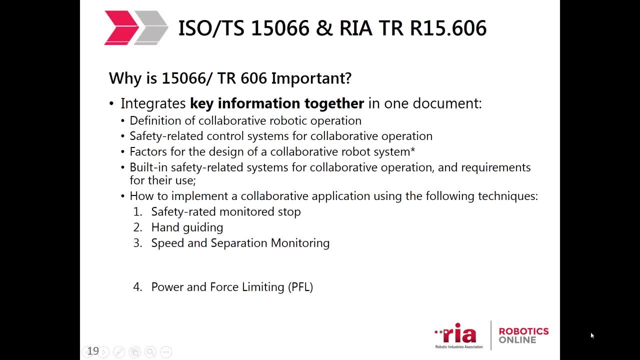 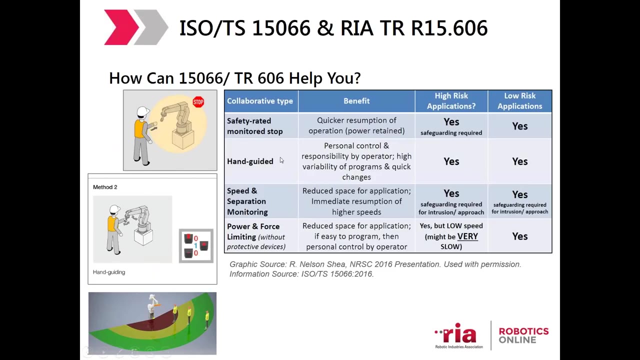 monitoring and the most common power and force limiting, otherwise known as PSL, cobots, And everything basically shown in pink is what is new? information that was included in TR-606.. So we're not going to get into the details behind the difference. 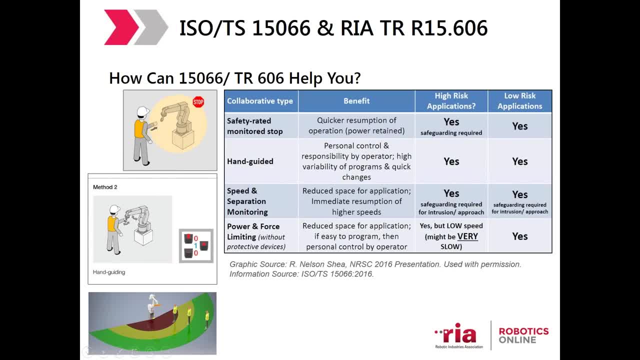 in these four types of cobots, just so you know that there are different types of cobots. So, again this chart, we're going to look at the four types of cobots And the first one, the one that was presented by Roberta Nelson-Shea. 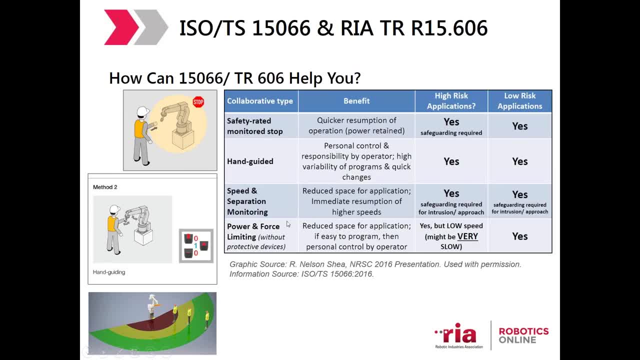 at NRSC and shows the four different types of collaborative robots- safety-rated, monitored stop, CAN, guided speed and separation monitoring and CFL- And their benefits versus traditional industrial robots. Risk assessments need to be performed on cobots And, depending upon the results of the risk assessments, 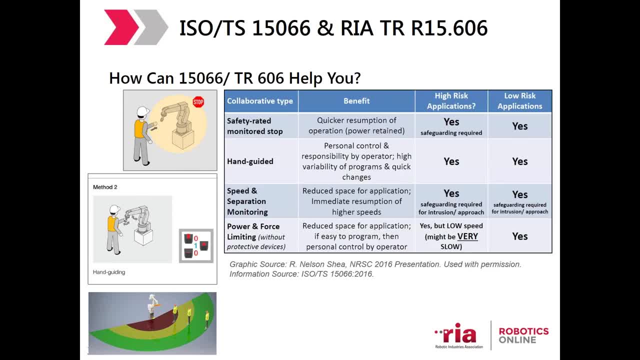 you may need to safeguard your cobot in high-risk applications. Confusion definitely exists on the topic of safeguarding cobots. In fact, the industry has not even settled yet on a definition of what is a collaborative robot. Most people using the term collaborative robot are referring 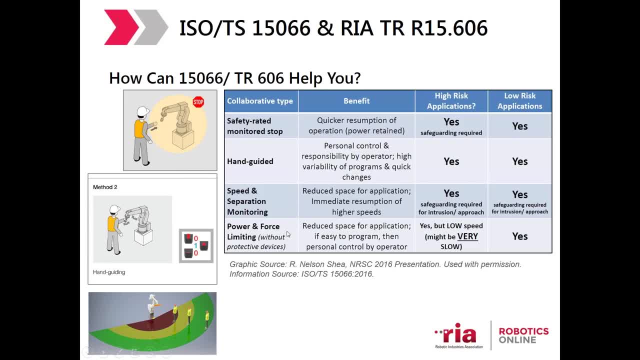 to what the industry standard prefers to call power and force limiting robots. But here again, power and force limiting robots is just one type of cobot. It is not the whole cobot category. But at the time that TSV was developed we had a lot of people using the term collaborative robot. 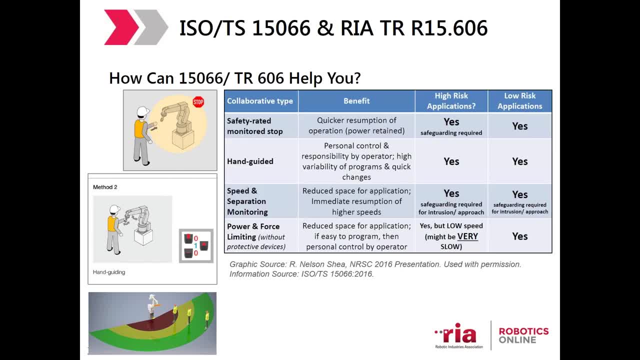 TS 15066 was being created and published. That was really primarily the only type of cobot around, And so there is confusion in this area. The PSL robots typically have most, if not all, of the following characteristics: Limited payload capacity. 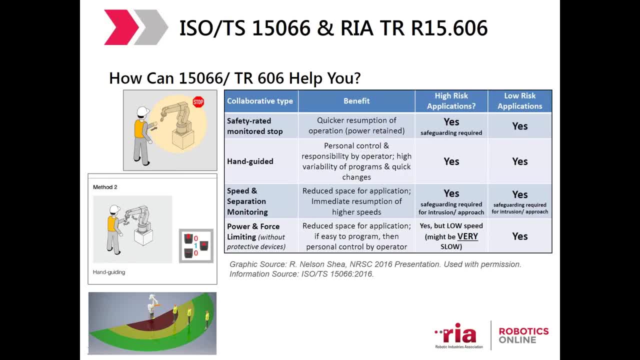 Limited size and mass of the robot arm, Limits placed on the pressure the robot arm can exert at its joints, Rounded edges and corners. Soft compliant surfaces, Easy to program, Integrate and move, Easy to hand, guide And more So. much of the buzz about collaborative robots is really. 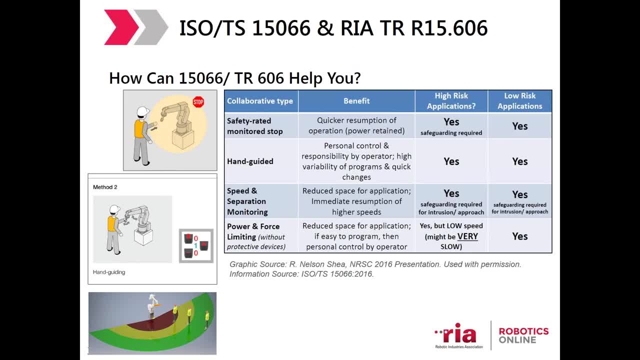 buzz on PSL robots And it is all about how this thing is safe right out of the box. Well, it may be the case that the PSL robot arm by itself is safe right out of the box, but this is not necessarily true about the robot once it has been integrated. 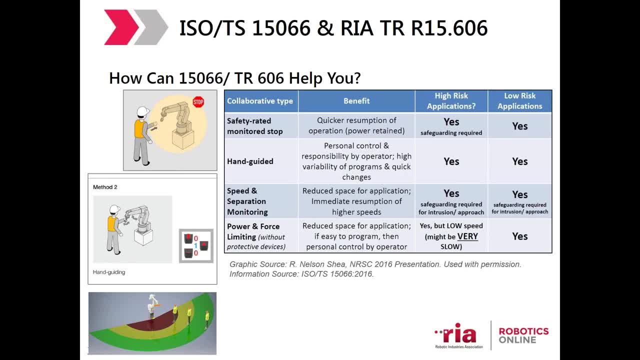 into a complete system. So understanding the application of the robot arm, the application and the operation are critical to understanding the need to safeguard. So remember that the robot arm by itself cannot do any work. It must be integrated with an end effector and other relevant 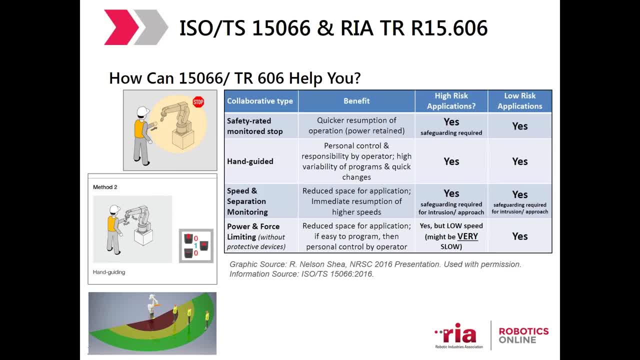 equipment and machinery in order to do a given task and a work piece, Which all must be appropriate for collaborative operation in order for us to say whether the overall robot system is collaborative. By appropriate we mean the power and forces it can exert are such that a human would not be harmed, even if incidental. 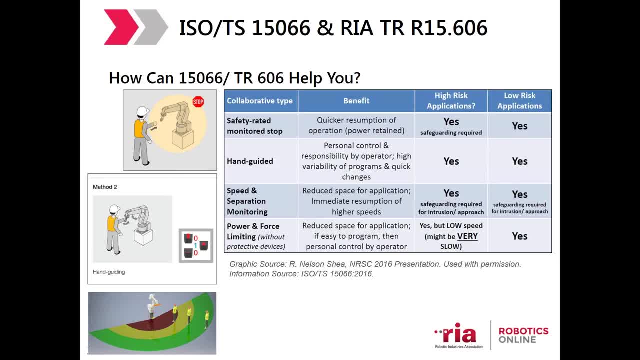 contact occurred, So I find this example to be helpful. So if the PSL robot arm would be juggling knives, that's not an appropriate application for a collaborative operation. Obviously that's dangerous. There should be other safeguards in place to keep the human 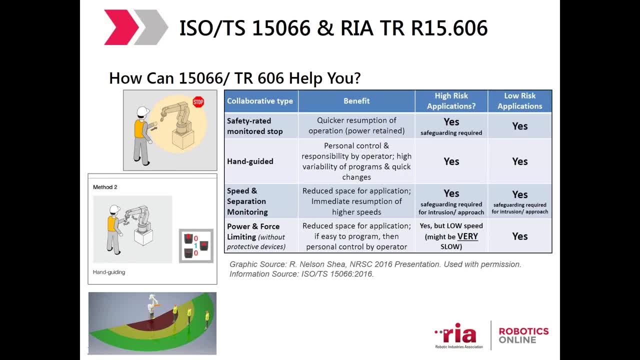 worker safe And those other safeguards are not safe. So the robot arm must be integrated with a traditional industrial robot, such as physical fencing, light curtains, pressure mats and so on. Or sometimes the collaborative is appropriate, but only at a low speed, because higher speeds would cause greater force to be. 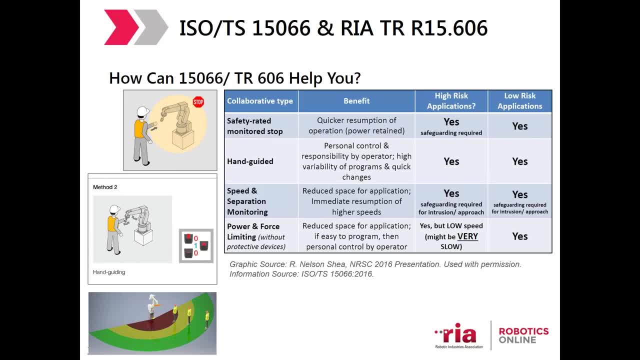 exerted at the point of contact such that the greater force exceeds the permitted force limits. If the user company would like the system to operate at faster speeds to enhance productivity, then PSL robots would need to be fitted with safeguards. So the bottom line is that it is really your risk assessment of the overall robot system. 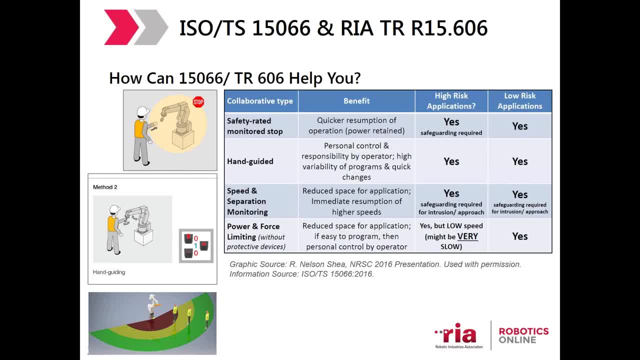 that will tell you whether or not the system is in fact, appropriate for collaborative use, even if it is using a PSL robot arm, And, if not, what safeguards should be put in place to protect the human workers nearby. And that's why a risk assessment is required, even for a collaborative robot system. 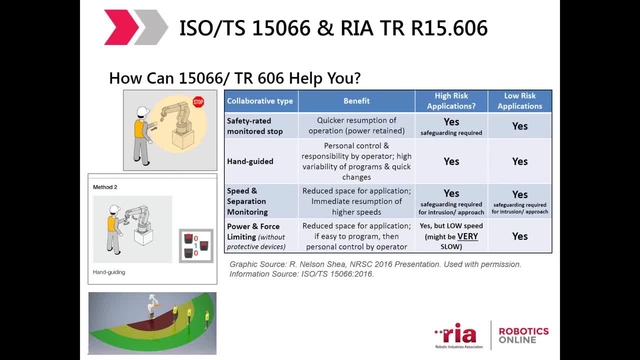 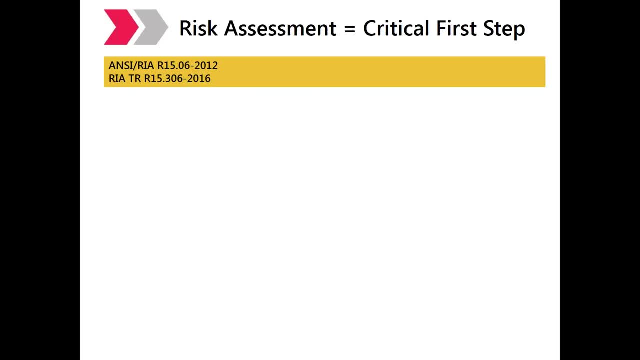 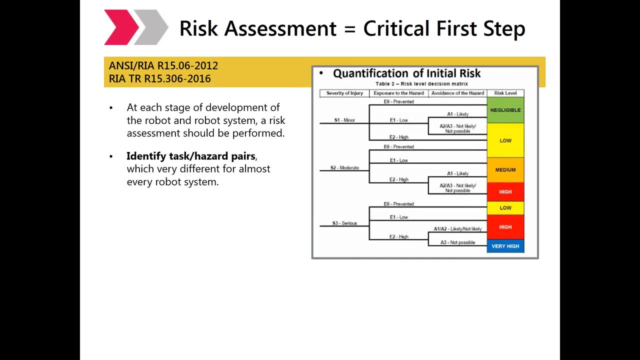 And remember, every situation is unique. So this slide just shows you a little bit more about risk assessment, which again is TR306.. And, by the way, you can purchase the standard R1506 and all of the technical reports over at the R1506 website. 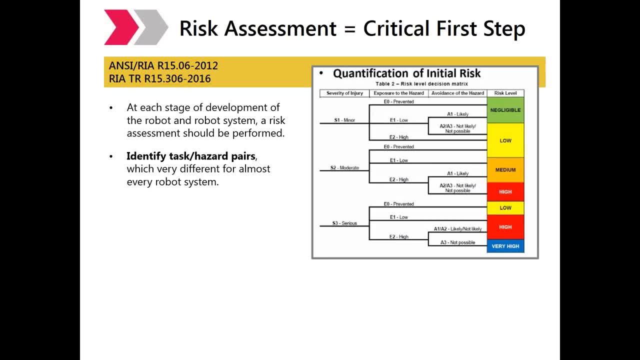 the Robotics Industry Association RIA website, which is roboticsorg. You can purchase them all together in what they call the safety bundle. So in TR 306, it describes a task-based risk assessment. So at each stage of development of the robot, the robot system, a risk assessment should be performed that identifies, not 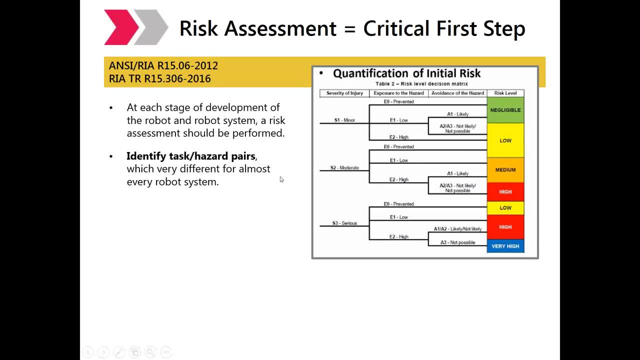 only the tasks but also the hazards, and then creates a task-hazard pair which would be different for every robot in the system, And then the appropriate level of safeguarding would be determined by what the risk assessment says. So the risk assessment is looking at the severity of injury, exposure to 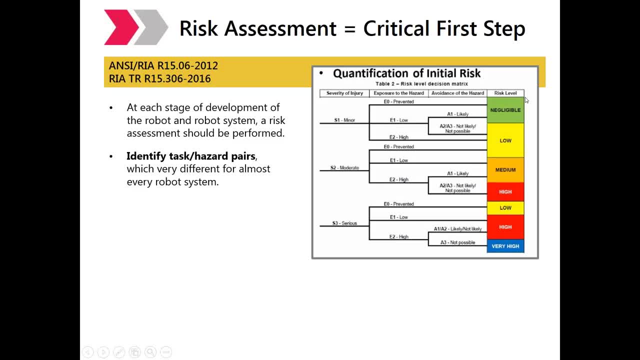 the hazard and the avoidance of the hazard, and creates these task-hazard pairs, which ultimately, then, will define the risk level. So, once the risk level has been defined, if it is high or very high, you may need to deploy some more aggressive risk reduction. 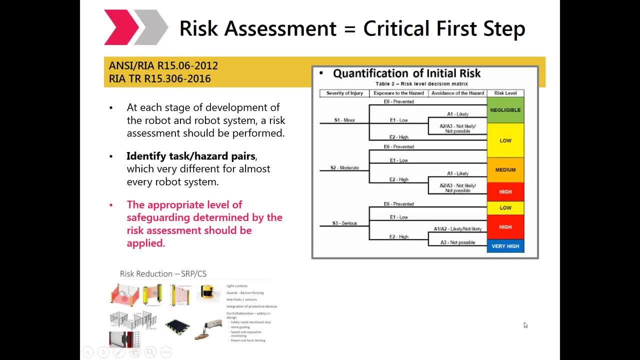 technologies such as like curtains, guards, interlocks and so on. If the risk level is low or negligible, you may need to deploy some less aggressive risk reduction solutions, such as signs or PPE or training. So it really all depends on what the risk assessment says. Okay so 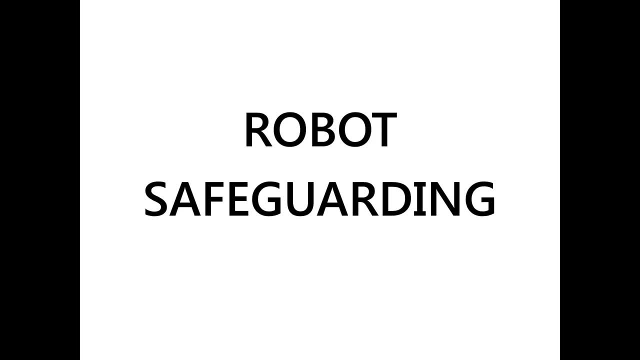 now I'm going to turn this over to Roger, who will get into some very specific robot safeguarding examples and provide some application expertise. Good morning, My name is Roger Harrison. I'm the Director of Training for Rockford Systems, So we do monthly training seminars here at our training center in. 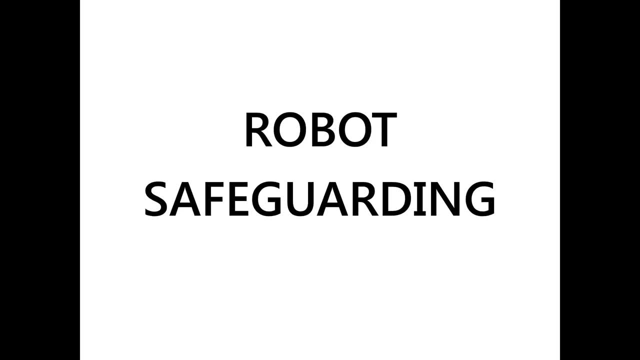 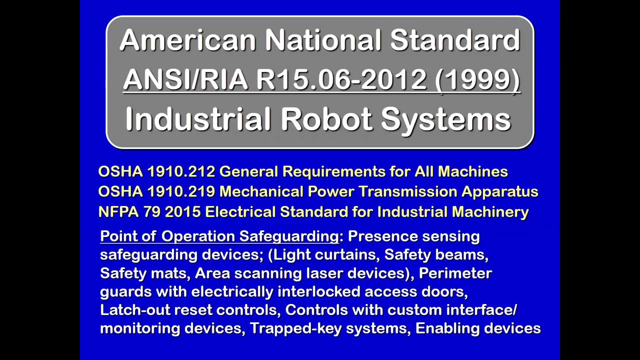 Rockford Illinois, as well as classes on the road and, occasionally, webinars like this one. I started with reading the 1999 Industrial Robot Standard R50 and R06, back then, and that's where I learned a lot about robots safeguarding techniques. 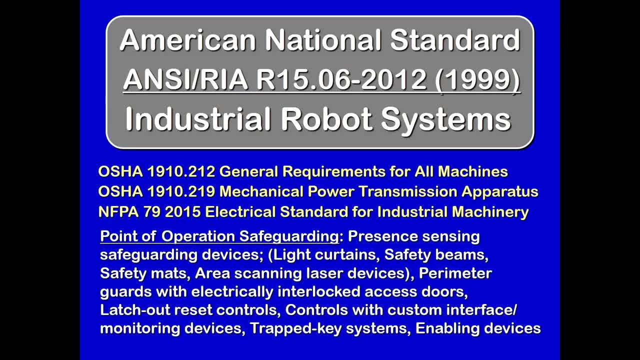 I think that was probably the most valuable of the standards that I'm going to mention that I used for their purpose and it is still available from the Robotic Industries Association about the 1999 version. that was updated in 2012 and it's a much larger document, most of which is on risk assessment. one way or 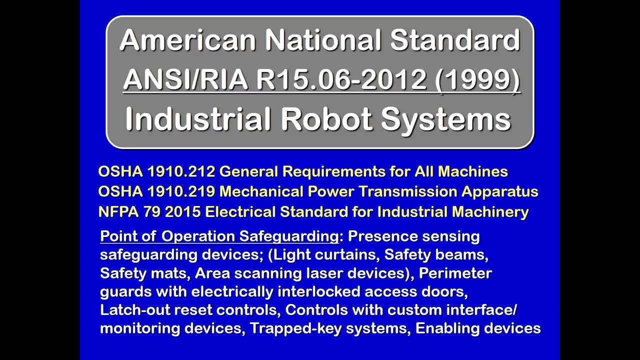 the other. there's a little bit on safeguarding in there, but I think the best update for me for this topic of safeguarding was the technical report TR 15- I'm sorry, TRR 15.406 2014: safeguarding industrial robots, because that is a. 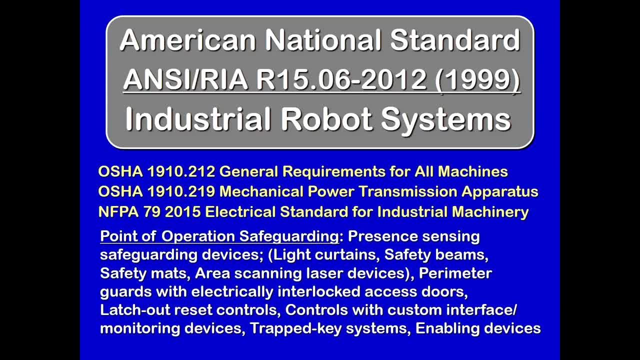 small standard again and has a lot of information on both guards and devices. if you want to just take the two main areas, if we look at the list here, they talking about fixed, non interlocked, interlocked and locking perimeter guards, because the basis for safeguarding a robot is based on a perimeter guard. 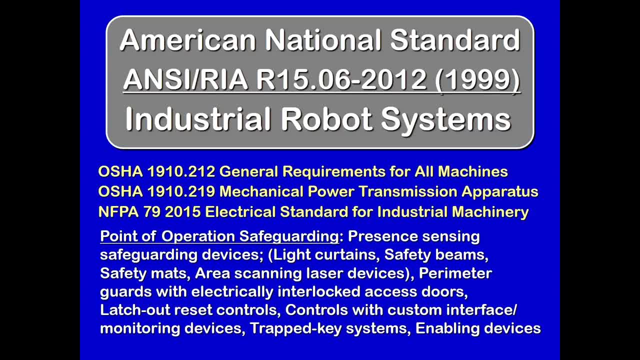 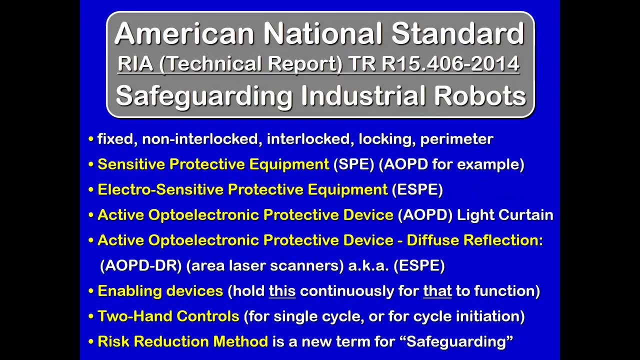 sensitive protective equipment. you've already heard that term this morning and what Terry Carver has described is that an ceremonies are. you know how protective equipment is designed: to protect your vehicle with a protective cover and it's broken down into electrical sensitive protective equipment, an active opto-electronic. 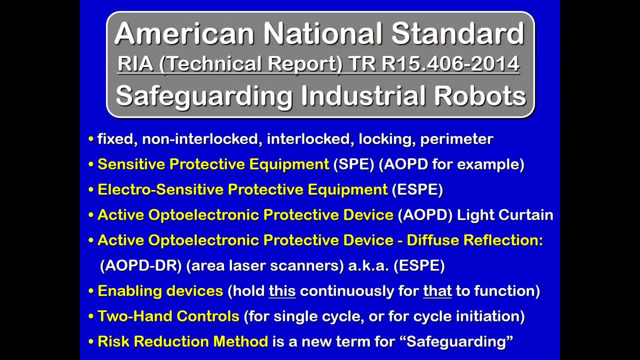 protective equipment, which is sometimes describes as as an active optical protective device, like a light curtain, and also applies to other machines like, for instance, laser devices on press brakes as an example. if you come further down, there's enabling devices, mentioned here, to single cycle the machine, because those are not used for safeguarding, and robots they now refer to. 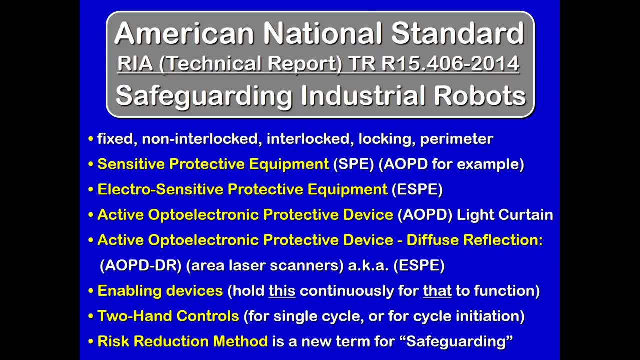 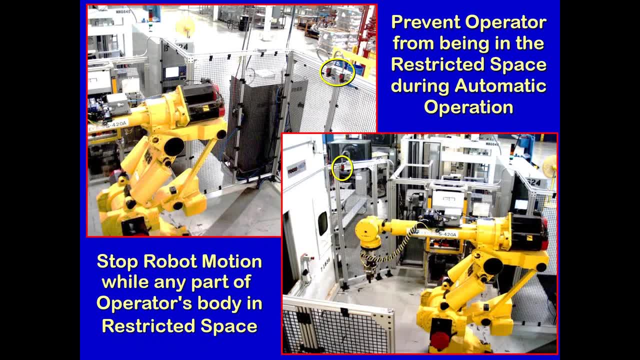 safeguarding in some places in this, these standards as a risk reduction method instead of using the term safeguarding- the two basic principles of safeguarding a robot, and these go back to the 1999 standard that I mentioned. our top left corner to prevent the operator for being in the restricted 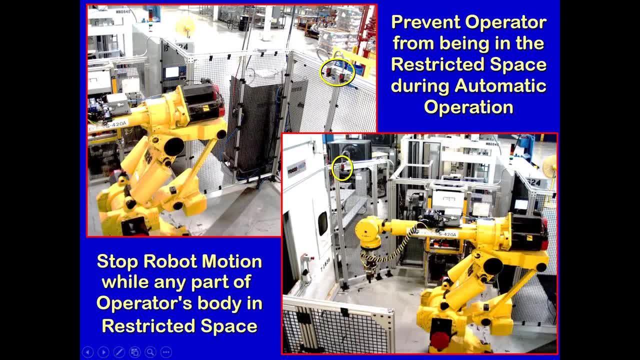 space during automatic operation. that's what the perimeter guard is all about and in the bottom left corner, stop the robot motion while any part of the operators bodies in the restricted space. those two things I'm guessing in looking at this robot enclosure are probably pretty well covered. 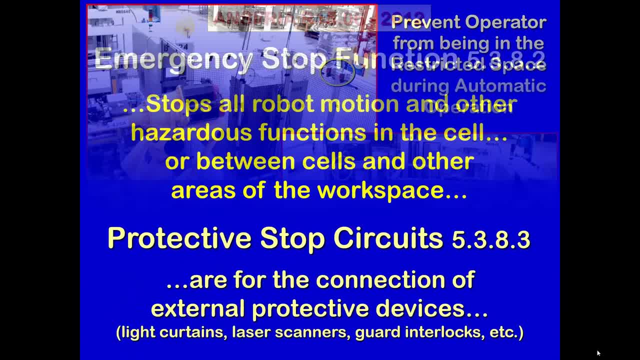 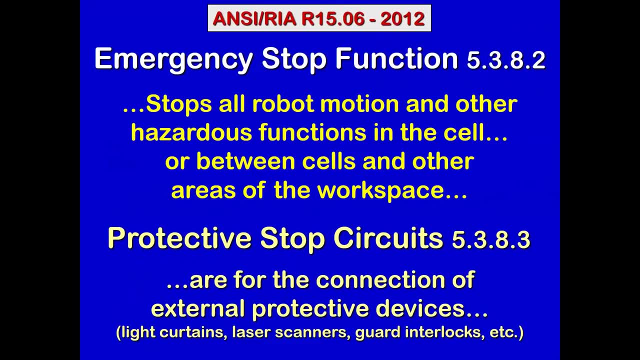 two different types of stop functions are defined in the 2012 standard emergency stop, which we're all familiar with. the stop only the robot motion and other hazard as a dysfunctions at the cell or between cells or other workers at the workspace. okay, we know about e stops- as opposed to protective stop circuits, which are for the. 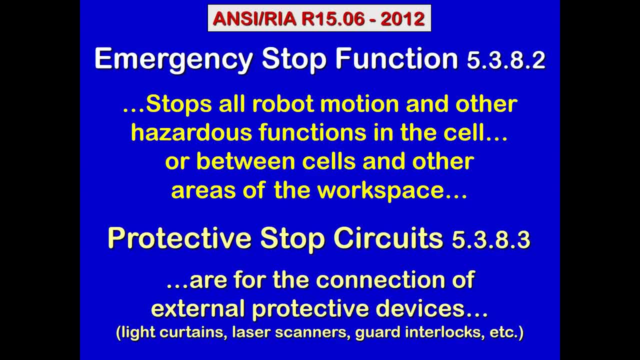 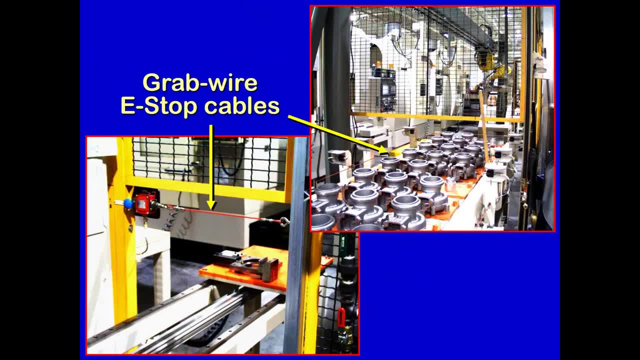 connection of external protective devices such as infrared light curtains, laser scanners, guard interlocks and so on. now, as far as cables for emergency stuff, also known as grab wire cables, those can be little short lengths, like you see on the left side, or much longer lengths lengths and go into an automation cell, maybe turn the corner with a pulley and go several. 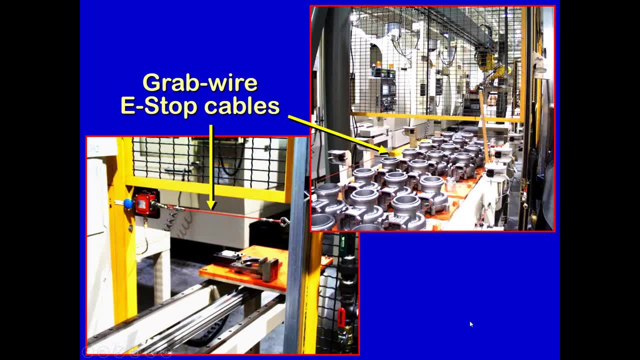 different directions before they terminate it the other end. so those can go quite a difference. I've seen it goes as far as 200 feet, as opposed to emergency stop buttons which are both more common on a lot of different machines which have to be. we're summarizing here several different 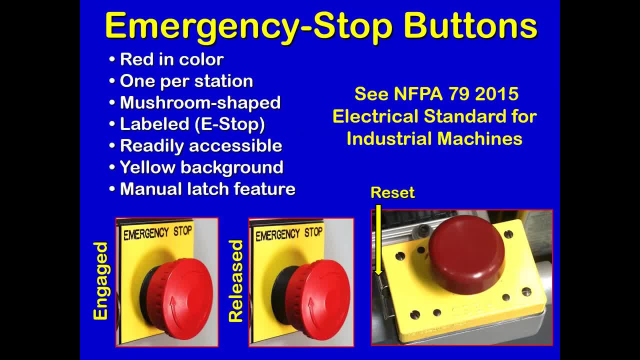 regulations or standards to say these: red in color, one per operating station, meaning if you have more than one operating station, need more than one red ever emergency stop, but a mushroom shape. you don't want little tiny red emergency stop buds with something that's a pretty good. 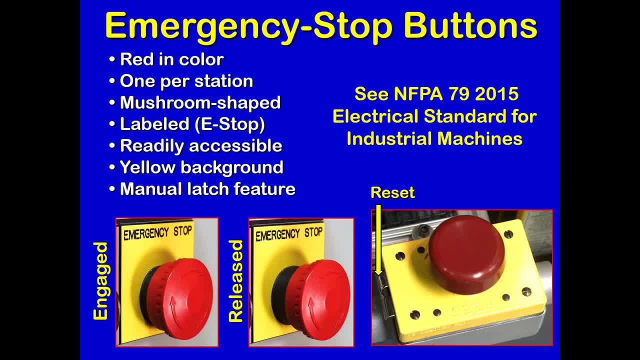 size. it's got to be labeled as a stop and be readily accessible to wherever the operator is working. and it could be more than one operator, meaning more than one stop. a yellow background is what indicates an emergency stop from any other stop and a manual latch feature. so when you push, 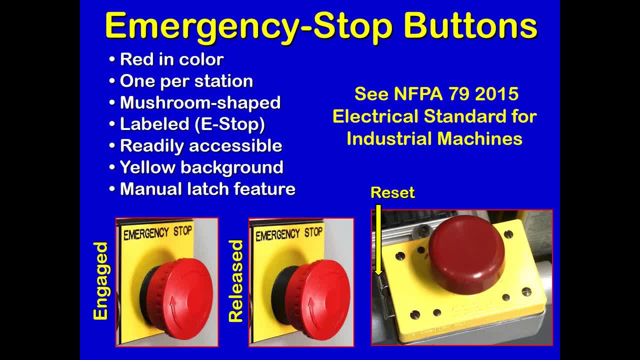 a button down. it latches in the engaged position, like the one in the lower left corner down here. to release it, in this case, you give it a quarter turn clockwise. it pops back out to the reset position so that you can go back to the regular controls to start up. 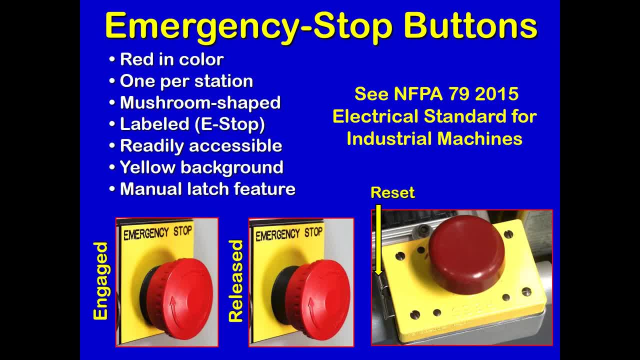 the machine or robot, whatever happens to be, and now releasing a red emergency stop, as I think we're all aware, does not initiate any hazard. this motion, the one on the far right hand side, is a little more heavy-duty. still the red button, yellow background with a manual latch. so when you push, 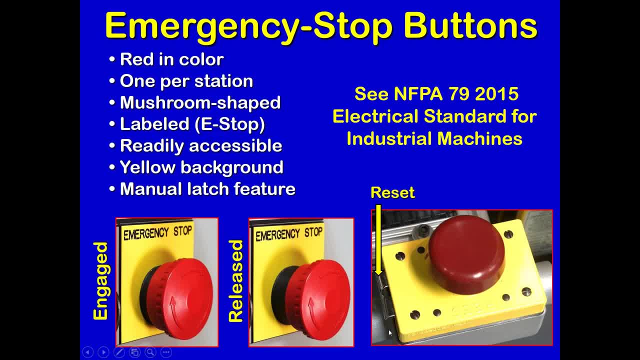 that button down, the latch pops out, so you can use that hole as part of your lockout tag out procedure. certainly not all of it. so the main safety standard- look at to see what we've summarized here- would be the National Fire Protection Association. 79 is the number of 2015, so latest. 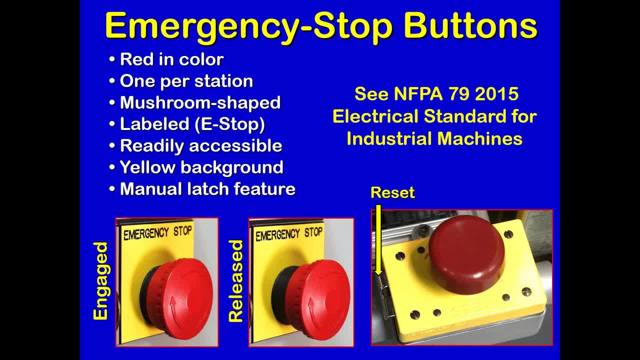 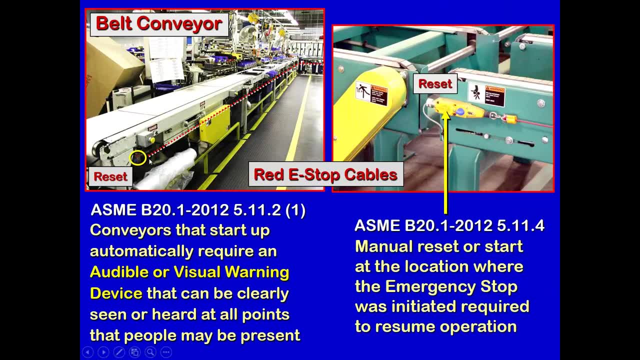 update. that's the electrical standard for industrial machines. now, grab wire cables can also be used on conveyors, which of course conveyors are also used with robots, as we'll see later. so you can exchange, or I should say exchange, but instead of using buttons, ready stop buttons, you can use cables that cover a long length. 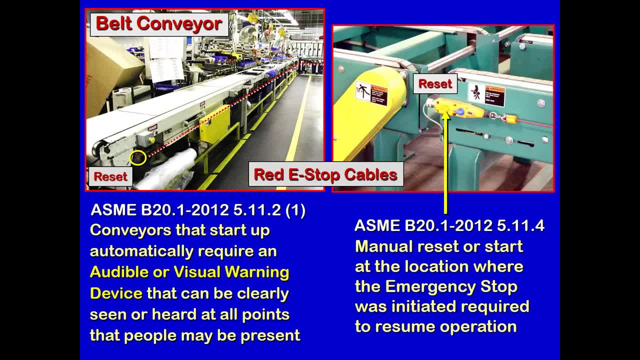 whether it's a conveyor or processing line where it might be notice. on the right side there's a reset switch and there are warning or danger signs that have little pictograms on drawings depicting what the hazard is. so on the left side, at the bottom- there they talk about conveyors- start of automatically requiring an. 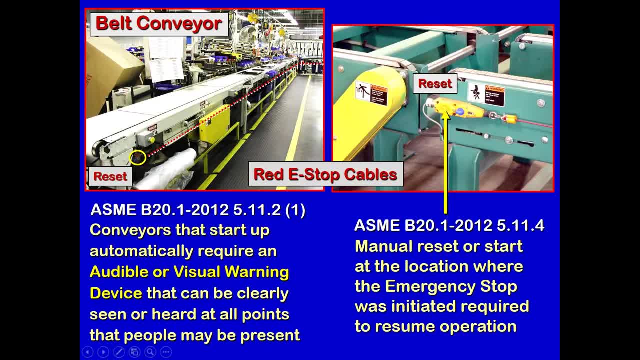 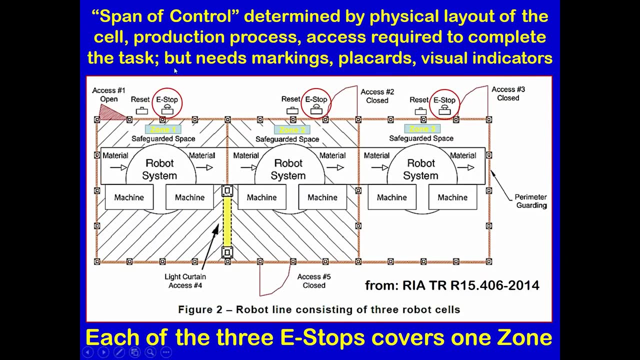 audible or visual warning device. span of control is a term used in that safeguarding technical report that I mentioned before. in fact this is taken from that report and shows three different span of control stop buttons: one of the top left here for emergency stop. one in the center right. 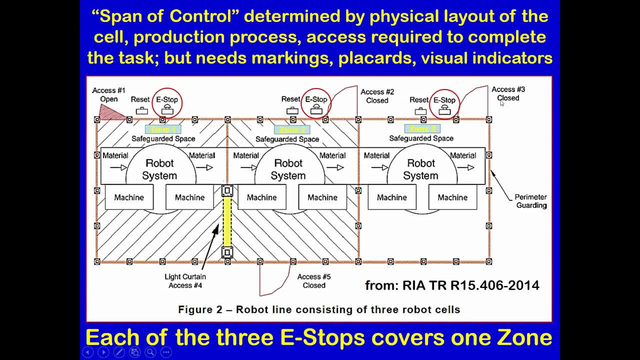 here and one over on the right side. if you press that, you're not going to use the sistem right there on the right hand side. so if that has to be, you look up the top here marked with placards or visual indicators to show what the span of control is for each of. 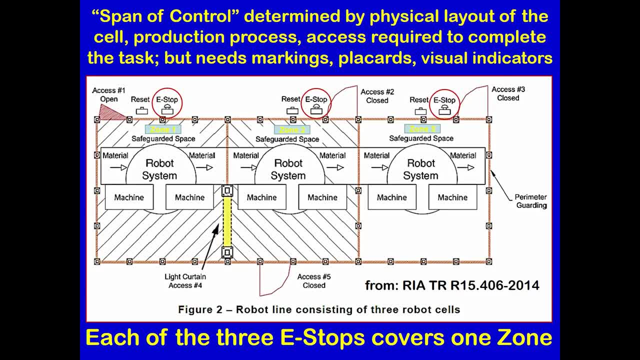 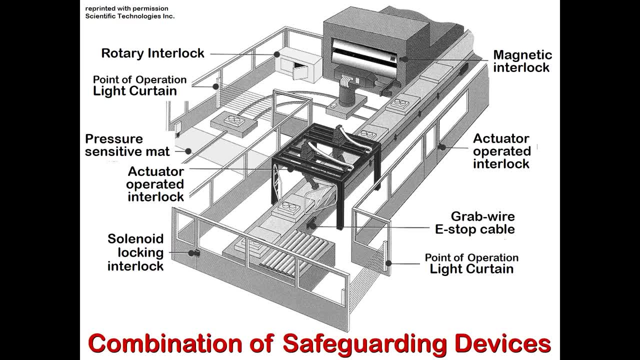 the three emergency stop button so you know what you're stopping when you hit that button. so safeguarding on robots is typically a combination of safeguarding devices. I say devices because that also includes the perimeter guard. it goes around the outside of it, which again is the basis for safeguarding, and 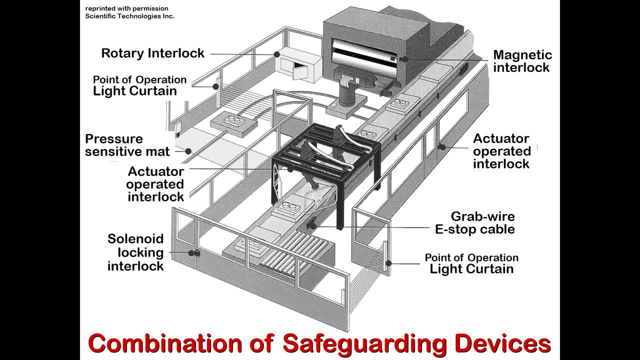 automation. so so we start with the light curtains. a lower right corner, there we have grab wire cables and moving up the side, here we got actual actuator operated interlocks, magnetic interlocks. over on the left side, here rotary interlocks, point-of-operation light curtains, pressure-sensitive mats, see 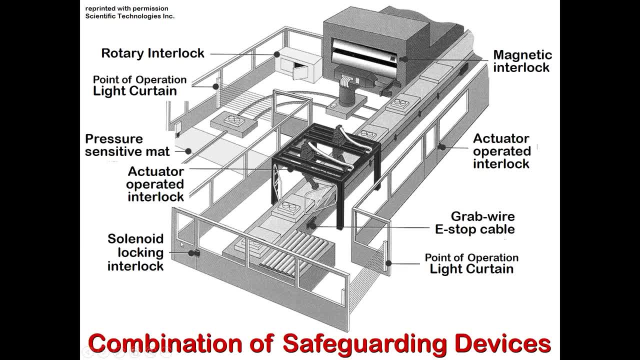 more interlocks, solenoid locking interlocks, and those need to all go back to some sort of safety input which in this case, the lower right corner, is referred to an output signal switching device. so if something's going along and automatic, all of a sudden it stops, you have to know which safe guarding or which stop. 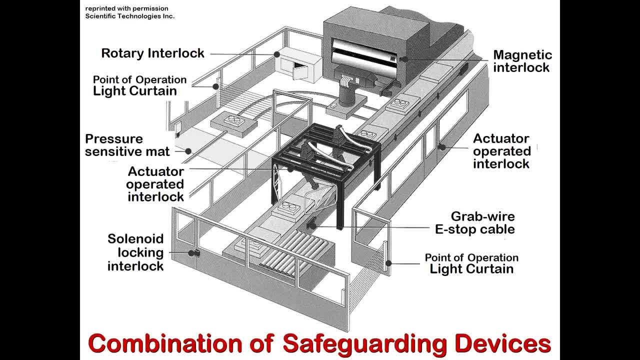 device to reset. in other words, did somebody accidentally step in the area where we have an area laser scanner? did they hit that emergency stop button or this one? did they open up an interlock door or break the point-of-operation light curtain? you really don't know, unless it gives you an. 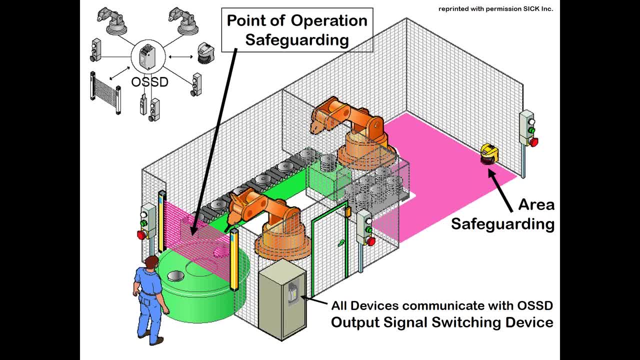 indicator. here we got another combination of safeguarding four different light curtains. that's two up at the top here for the conveyors to come through and two down on this side. we've also got two interlocked full body access doors, one on each side. we've got area laser scanners in each of the four. 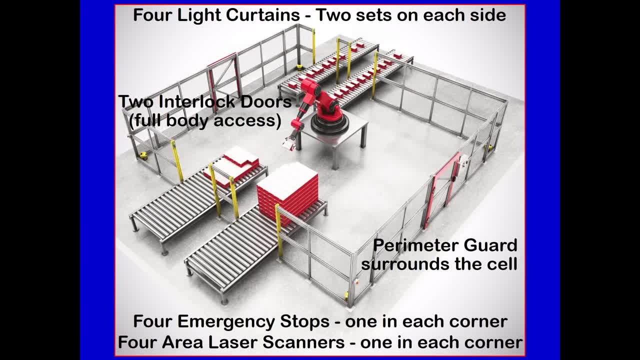 corners. now it's significant that everything that's inside the safe guard space is mounted on something with skinny legs because, remember, when the laser reaches out, it leaves a shadow behind it, and skinny legs do not create as much of a shadow as, say, the base of the robot dead. it were modern on the 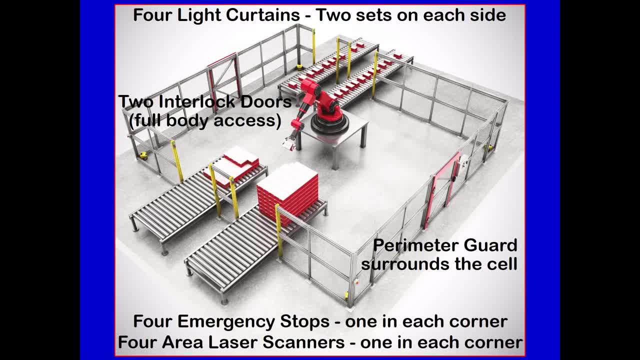 floor in order to let product in and out of that safeguarded space. yes, they can use a light curtain like this. some companies elect to use a guard with a smaller at the bottom that allows for the product only. but what if the dimensions of that load vary from one? 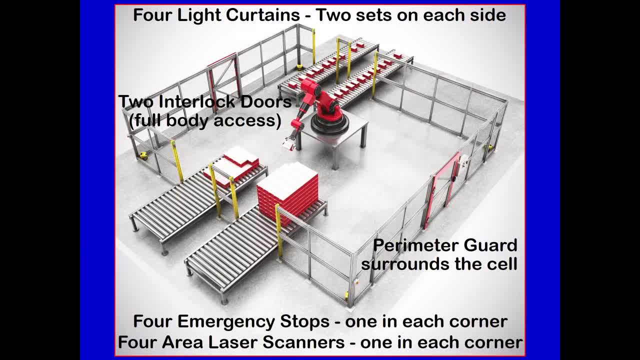 job to another. well, that's where we've installed- and I don't have a picture of it here- a sliding vertical guard from slides up and down on the track, meaning you can adjust the size of the opening underneath it. other companies have fabricated a tunnel for the product to go. 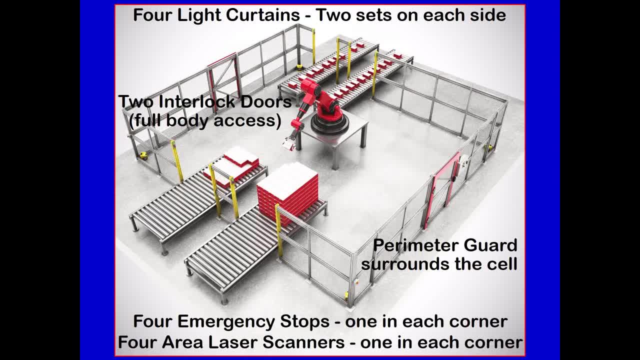 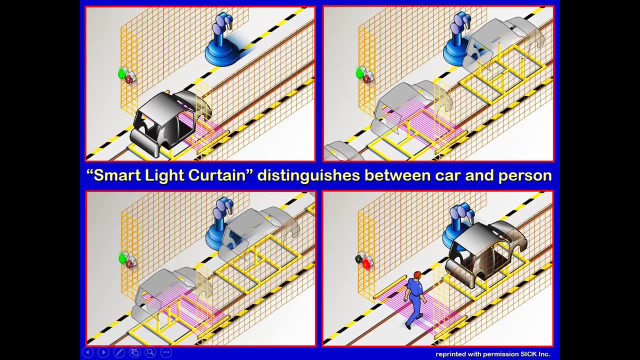 through, but again that's usually limited to something where you always use the same size product going through. there are smart light curtains- been out there a number of years now that could distinguish the difference between the car body going through this horizontal light curtain, like the top left corner, versus somebody walking through it like the one down here based. 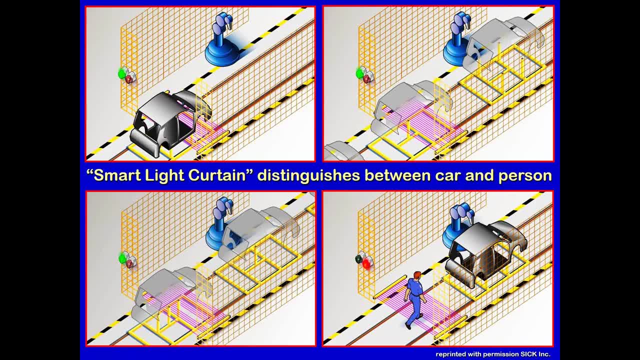 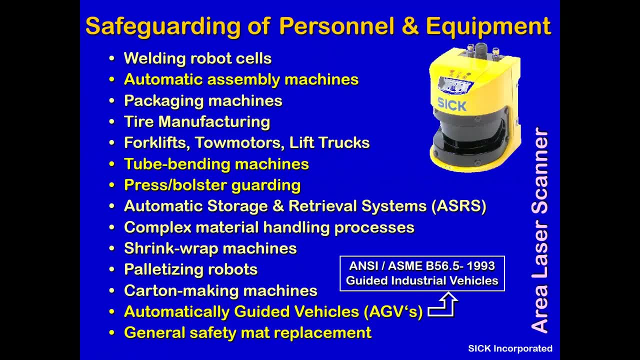 on the pattern of beams that's broken. smart light curtains, area laser scanners have been around since 1994. I think sick automation was the first one to manufacture these. there are other companies that offer these as well. let's say: we've got sick, they've got. 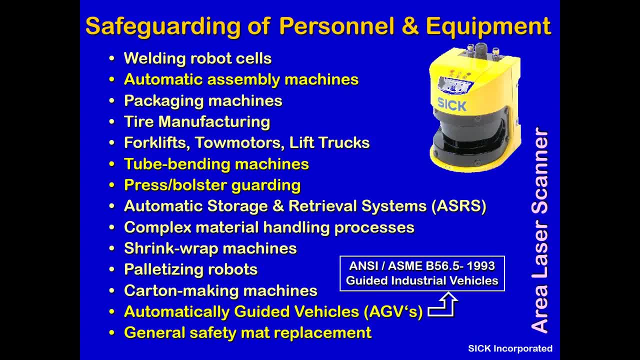 Omron STI. they got Keyence, we got Banner- are four of them that I'm aware of. I've highlighted some of the ones that I happen to have seen out there, like automatic assembly machines at the top, like horizontal tube benders, press, bolster guard. I say bolster guarding on a press because actually this: 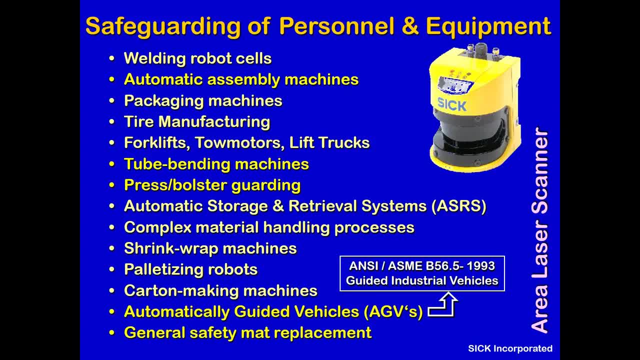 device is not a high enough safety category to match a safe category for a light curtain that's used for point-of-operation safeguarding. this is only, you know, one category underneath that, and the reason for that is both the transmitter and receiver. we are in one housing, which is not the case with light curtains, and we go down to the bottom. 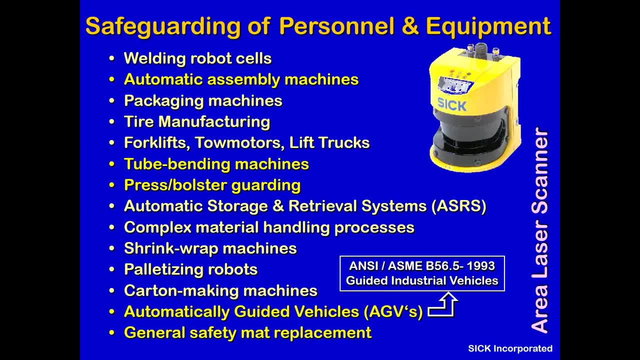 automatically guided vehicles is where this all began. AGVs- which, by the way, do have an ANSI standard of their own right here. and then general safety mat replacement. a lot of pressure sensitive masks get damaged by for trucks and chemicals, and so these are usually tucked away a little smaller. 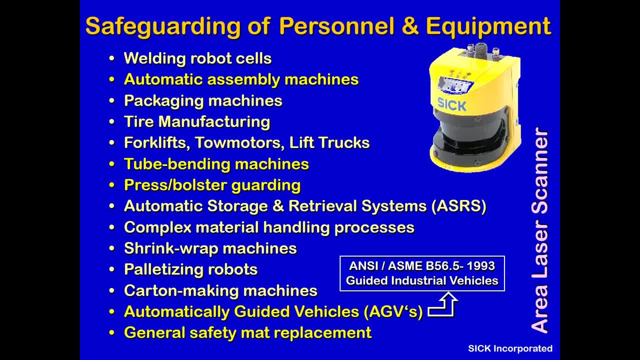 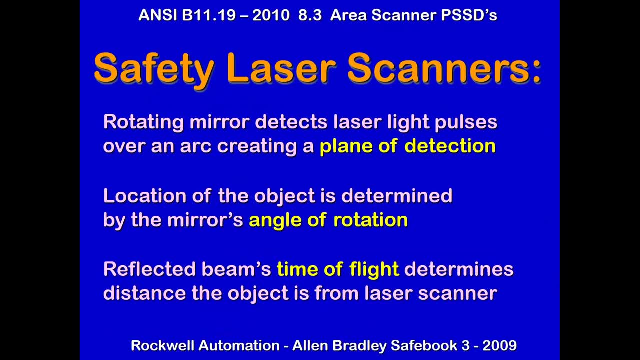 target for things like that, not that they can't be damaged. but you got to remember these are reprogrammable with your laptop out on the shop floor so if your parameters change, it's easy to change your parameters on an area laser scanner- three terms you hear a lot with area laser. 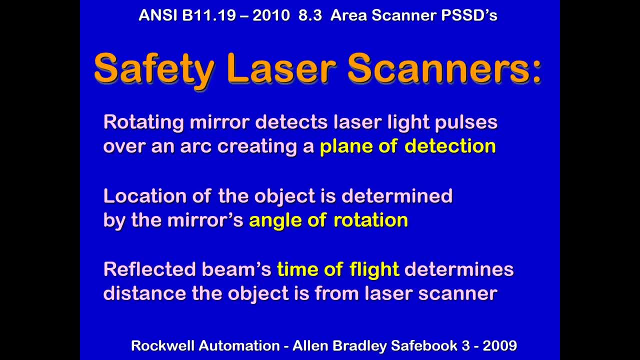 scanners, and that's your produce. safety laser scanner, and that's your. safety laser scanner- or floor scanners is another name, for one is a plane of detection which is usually somewhere between ankle height and shin height. they mount these so that people can't sneak underneath them. angular rotation goes anywhere from 180 degrees to 275 degrees, depending on what it was manufactured. 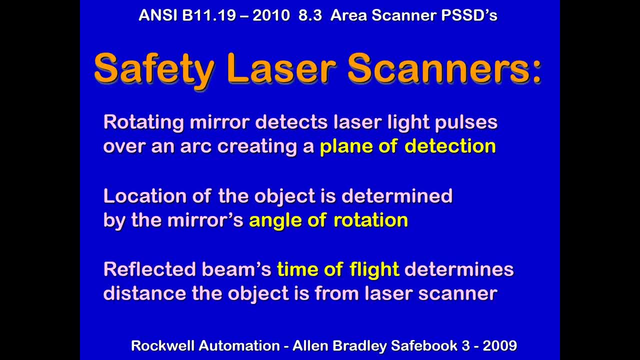 to be. there's an angle of rotation. you can even put two of these back-to-back to get a full circle. that's why they overlap with each other. you can even put two of these back-to-back to get a full circle. that's why they overlap with. 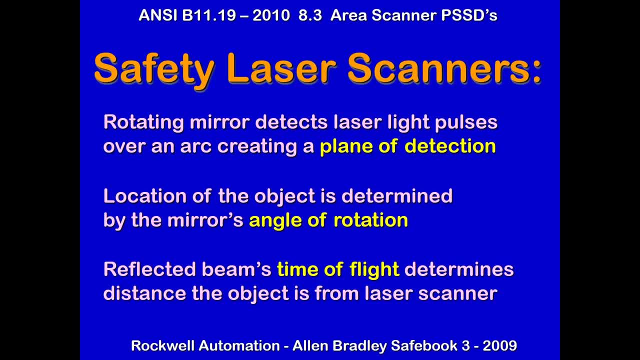 you can even put two of these back-to-back to get a full circle. that's why they overlap with the person with the angles a little bit. angle of rotation: let's see time of flight: when the laser itself leaves this device, bounces off an object and comes back, determines the distance away that. 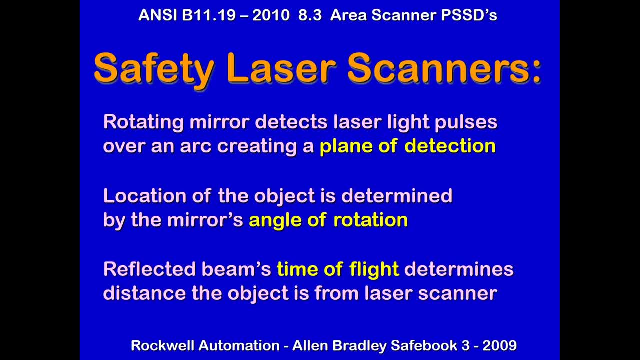 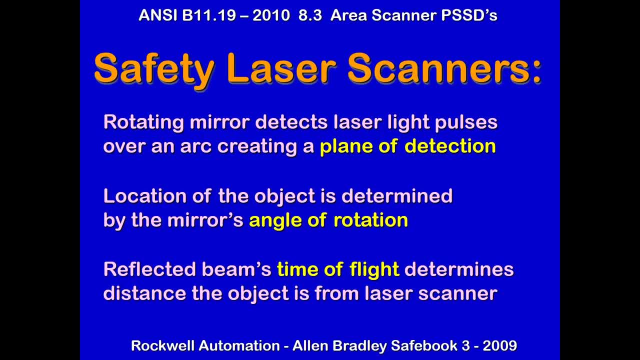 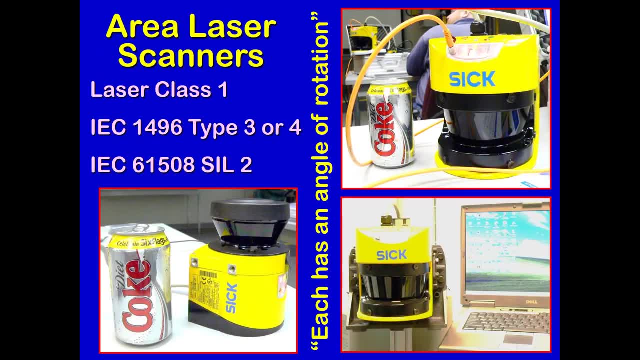 floor lining this thing up. you wouldn't, you know, be bothered by this laser hitting you in the face, even sweeping across the eyes, because it's such a low category. it's an IEC type three or four. now I don't think I might check this out. I don't think there's any category fours, only threes out there. 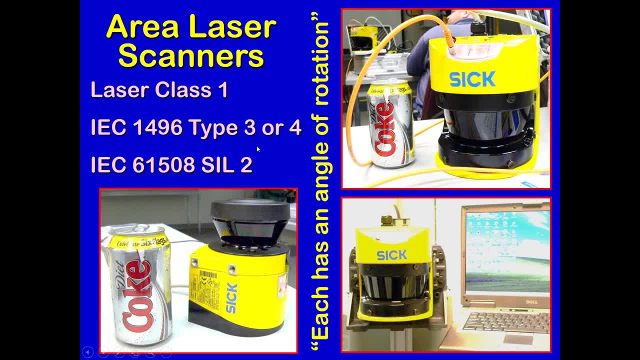 because of what I explained before, both the transmitter and the receiver and a one enclosure and to be a category for, like some of the light curtains, are you got to have a separate transmitter and a separate? you see the two separate enclosures. there's a lot of different things that you can do. 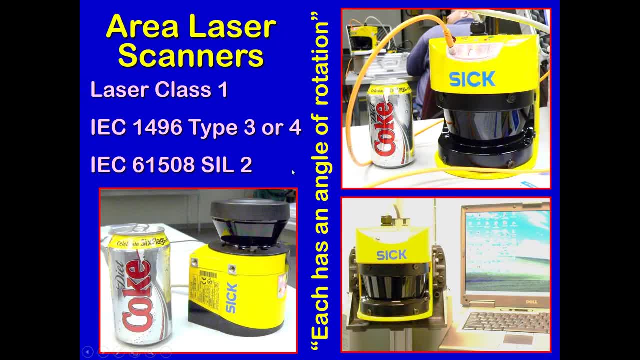 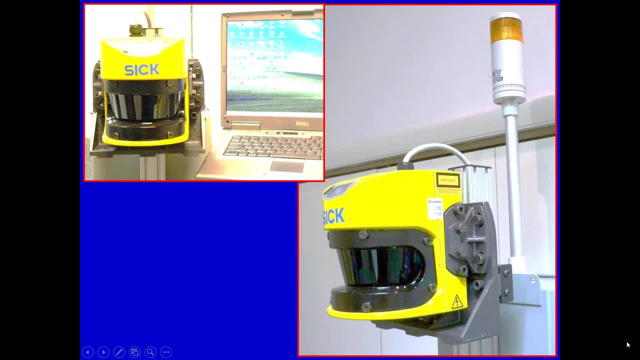 the safety integrity level is only a two as compared to, let's say, you have three on a light curtain. so these, compared to light curtains, which a lot of people ask us about in our seminars, require more safety distance than a light curtain because they don't react as fast as 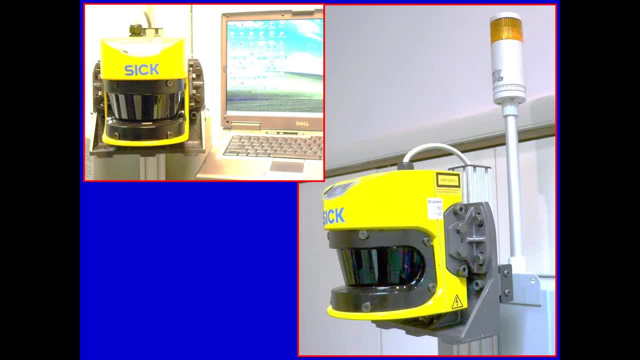 their reaction time again. the category is lower the sill level and they're two to three times more expensive than light curtains. so there are limited applications with these especially. we are talking point of operation safeguarding. so here's a laptop you can program and, as I said before, reprogram if your parameters change, right out on the shop floor with. 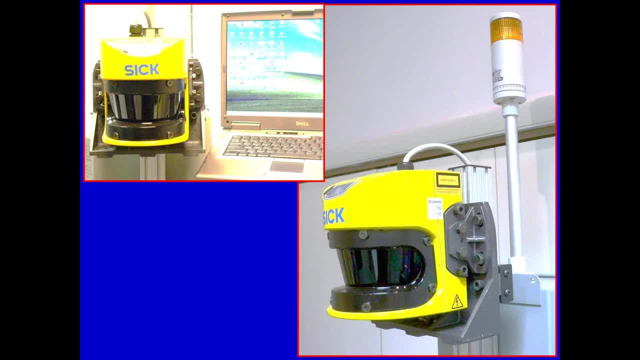 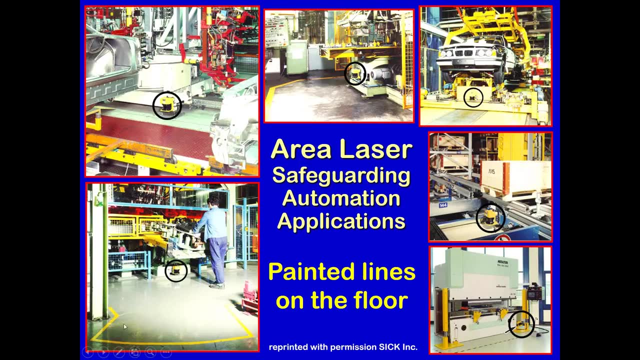 your laptop. they began in automation situations like you see here. some of these go back to the nineteen nineties. notice like, for instance, at the lower left here they painted a line on the floor where the pattern actually comes out to off the laser scan. so you know not to step. 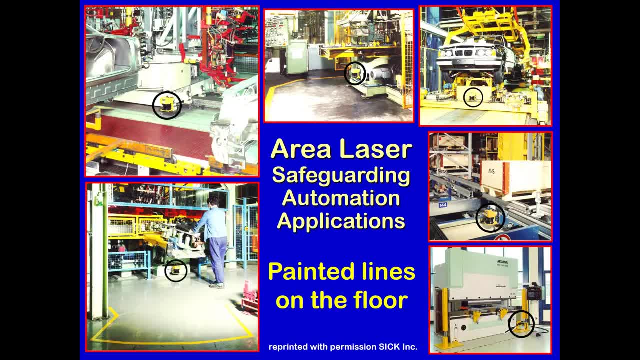 inside of that and accidentally trip the system. but the top center. there's another one where the floor line was painted. here down in the lower right corner you've got area laser scanners being used in conjunction with vertical light curtains on a bending break, press break. so basically you've got two applications: that area guarding, like you see on the left side. 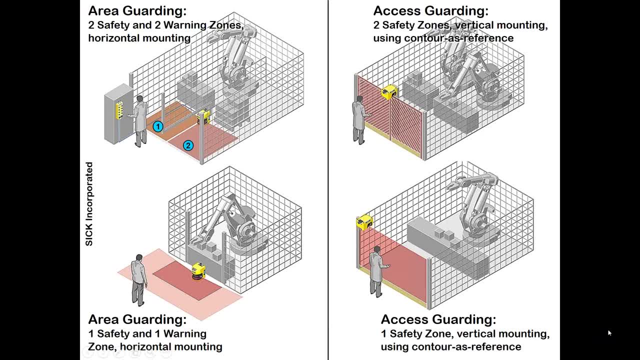 and access guarding like to see on the right side the most. most of the applications that I've seen are on the left side with area guarding where they're horizontally mounted, like the one down here in the lower left corner. now the dark shadow represents the fault zone, the light 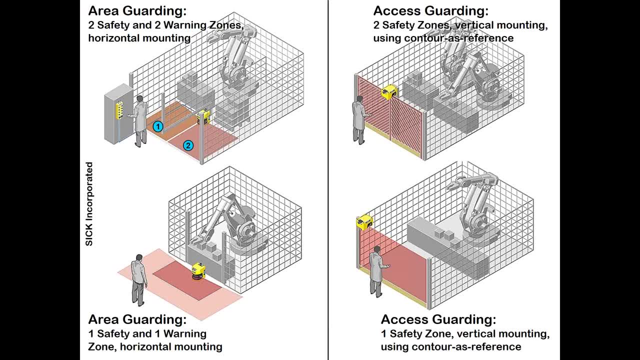 shadow represents the warning zone, which, in the case of this laser scanner, the fault zone can go out as far as 13 feet. the warning zone could blow out as far as thirty nine feet. so the operator steps into the warning zone, it flashes a light or beeps a horn to warn him. 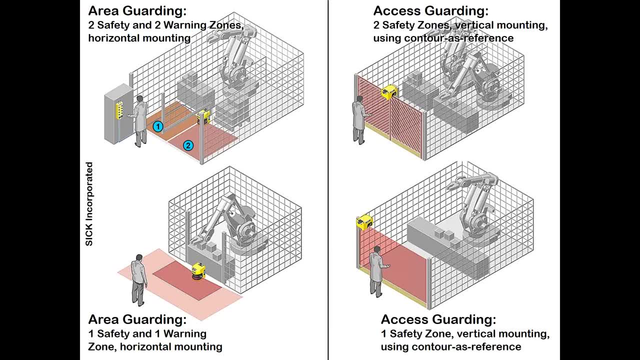 he's getting in there and slows the robot down to a slower speed. he continues and gets into the fault zone- the darker shading down here- that sends a stop signal to the guarded robot. so two different zones you can adjust and know it does not have to be a rectangle or a semicircle, it can be a lot of. 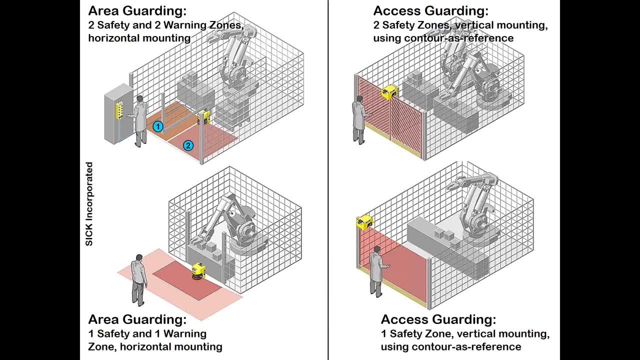 different patterns. the one at the top is similar but there's two zones. it's actually split with an a and a b zone. the one on the right hand side for access guarding notice. this is mounted vertically and, as i said before, more safety distance required than a light curtain because 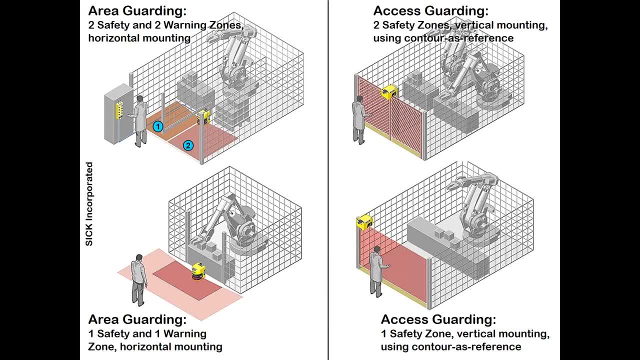 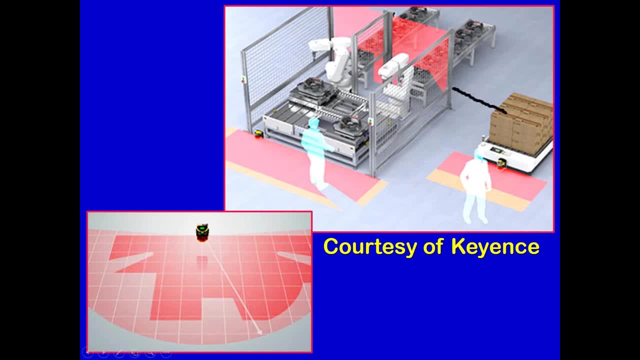 it's a slow reaction time. it's a lower safety category. therefore some machines like power presses for instance. they cannot be used as a primary safeguarding device, whereas a light curtain could, and they're two to three times more expensive than a good category four light curtain. 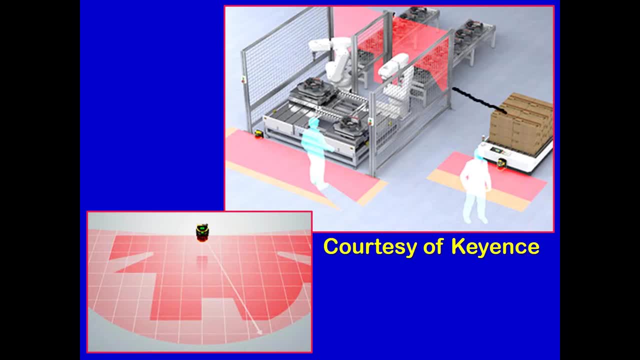 i say category four because that's usually top of the line. you're talking about light curtains. that's a key area laser scanner. right here you can see the dark shading is the fault zone and the light shading on the outside edge is the warning zone. so you got to think of an area laser scanner is like a bicycle. 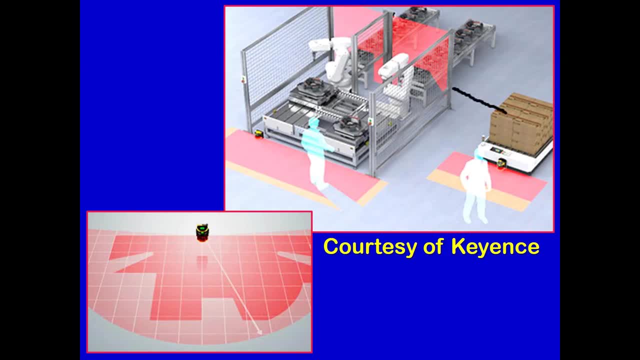 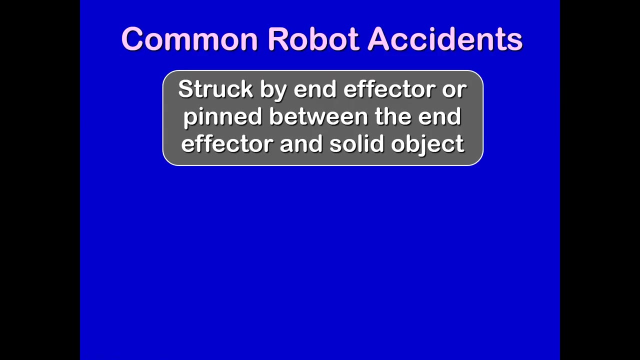 wheel starts in the center, where the spokes are close together, and the spokes get further away the further out you go. that's how it's designed. common robot accidents: people getting struck by the end effector or a pin between the end effector and a solid object is the reason for uh, the 20. 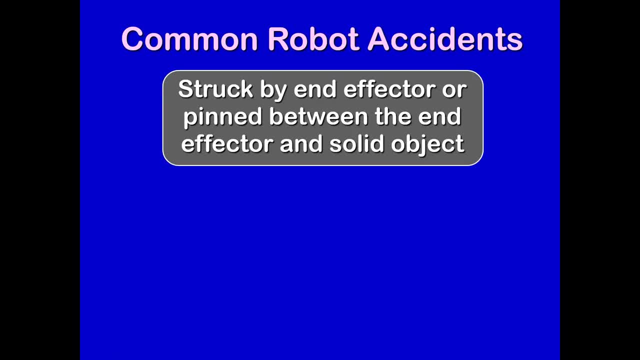 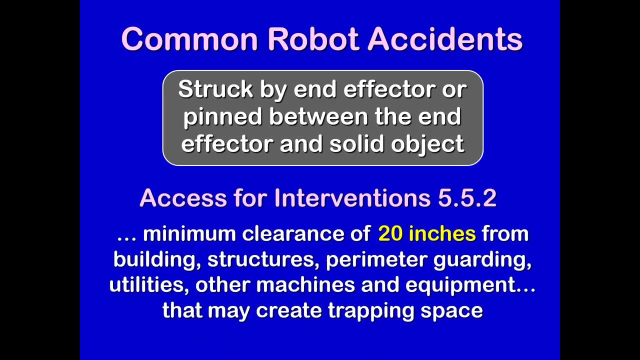 inch rule used to be the 18 inch rule when the robot arm stretched fully out as far as it could go to the end of the end of vector. i might say you need at least 20 inches clear from any solid object that could squash somebody. that's based on studies done in sweden and japan. 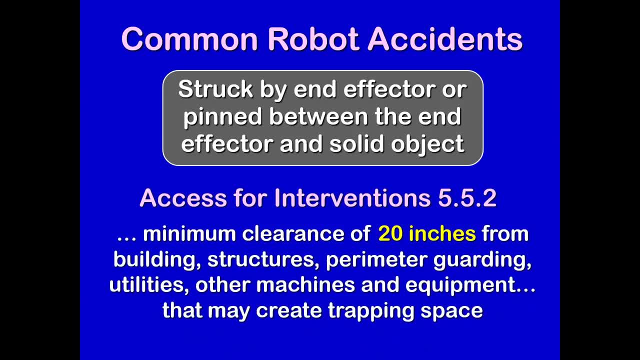 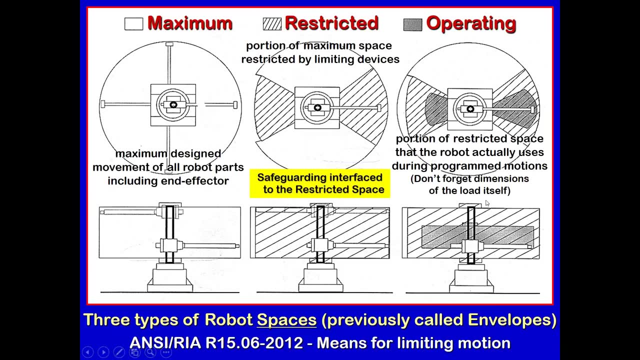 years ago, so the 18 inch rule has become the 20 inch rule. you'll find it under clause 5.5.2, under access for interventions. remember that the word envelopes the robot used to have three envelopes. now they've changed your name to robot spaces, you've got maximum. 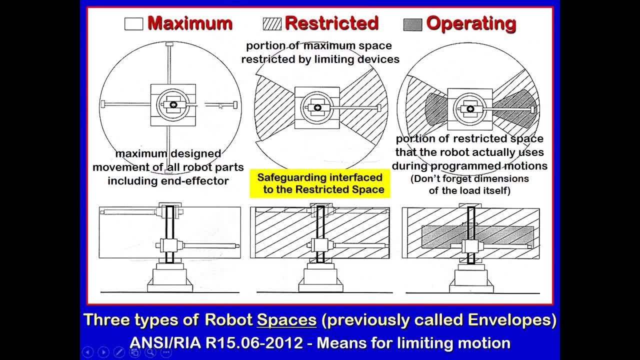 restricted and operating maximum is all possible movement, including the end effector. restricted is that portion of the maximum space restricted by limiting devices, which we're going to go on to discuss, because limiting devices are actually part of the safeguarding and, on the right hand side, the operating space is that portion of the restricted space. 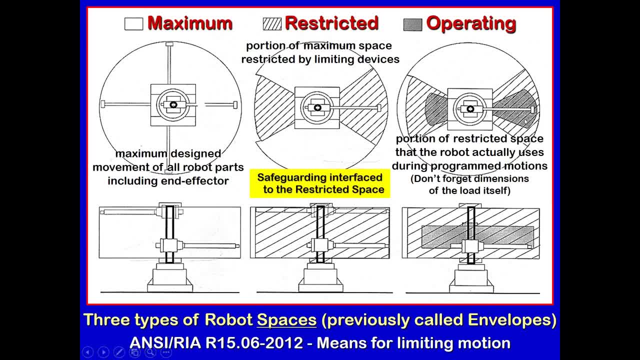 the robot actually uses during its programmed motions, not forgetting the dimensions of the load. by the way, notice in the center in yellow. here the safeguarding is usually interfaced to the restricted space, the middle one now, limiting devices. what are they? well, again, it's under means. 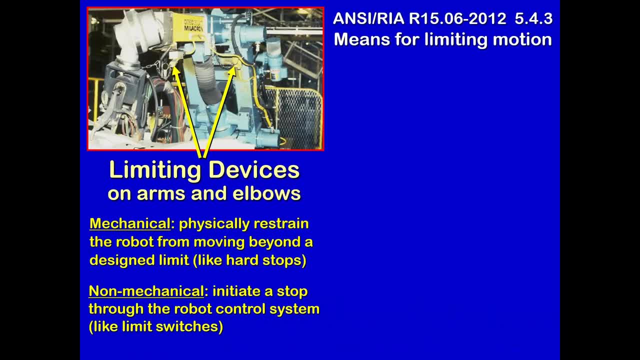 for limiting motion and there's two types. you've got mechanical limiting devices, like hard stops on the base or waist of the robot, and you got non-mechanical devices like uh, for instance, the pull plugs on the arms and elbows here. so if the robot goes beyond its restricted space, it's a 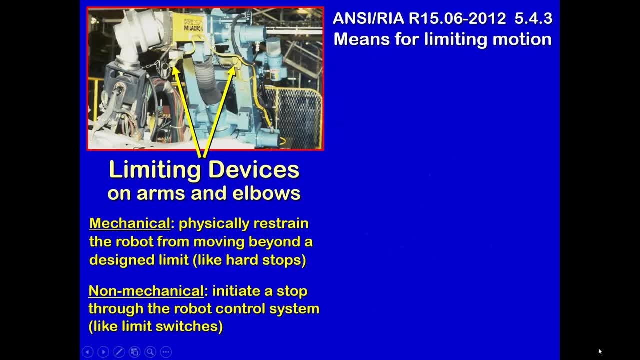 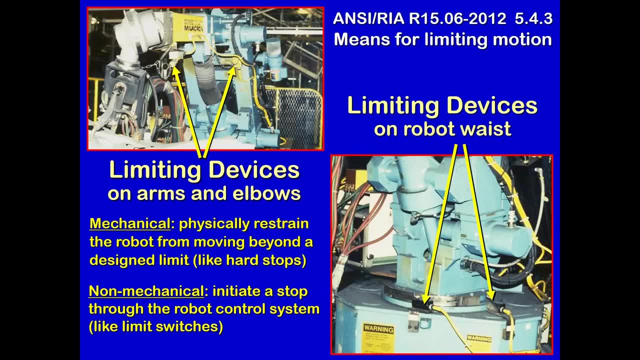 middle one remember- pulls the plug, cuts it by power, stops a robot. um, people think, well, i've got a hard stop on this thing, it'll stop anything. uh, no, no, i won't. i've heard of customers in our seminar to having discussions among themselves how their six-axis robot blew right through. 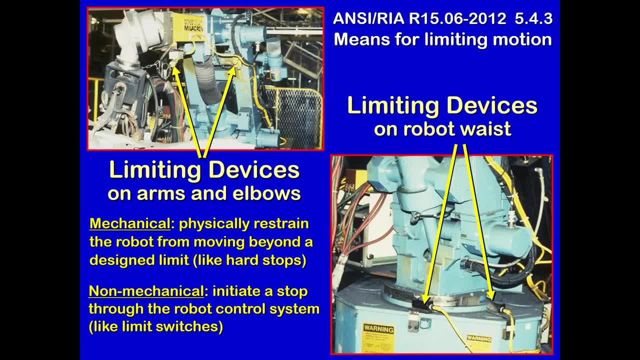 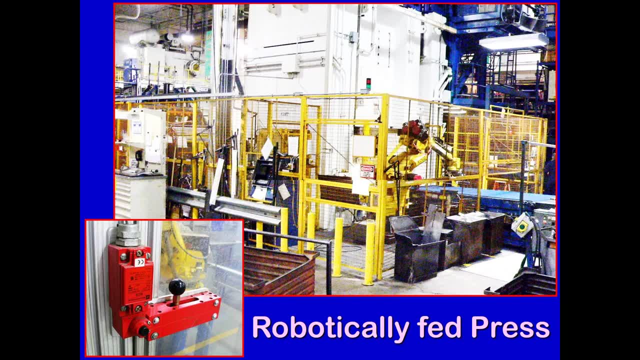 a hard stop. so you know, don't think those are the end all with that. robotically fed presses. yeah, here's a fence perimeter and, uh, there are interlocked doors to get in there. i'm not sure what's around the other side, but you see the robot right in the center here. this was a john. 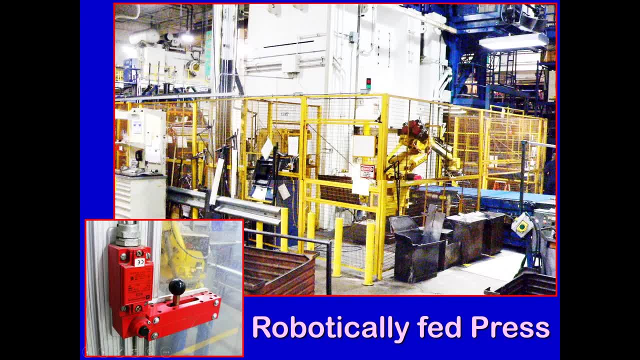 deer plant where they had robots on both sides, one to feed a rectangular part into the press press made one deep draw head and produced a mower deck, a riding mower deck, which was removed on the other side. so, going back here, you see we have a fence perimeter around it which 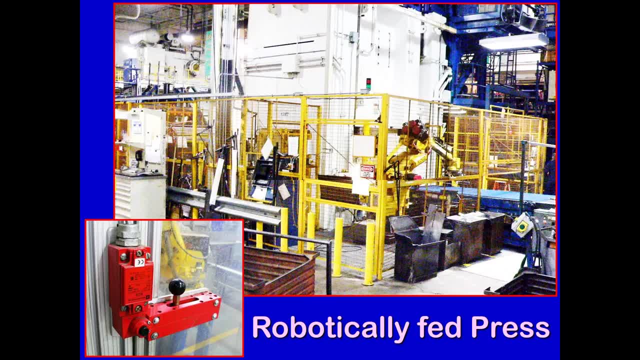 met all the requirements for interlocks and so on. um plus, when somebody had to manually be in there. if you look very closely here, there's a series of light curtains right here, sort of an l shape, to give you protection if you had to be in that space inside the fence. 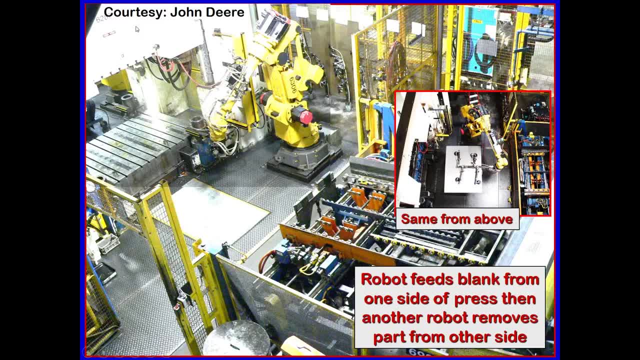 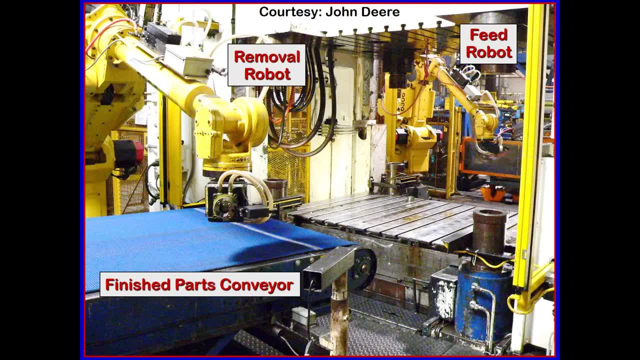 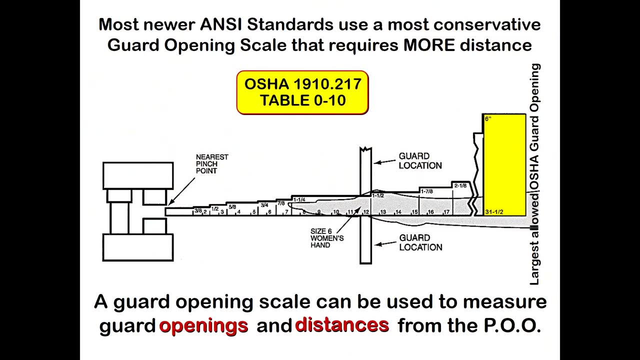 and there's your removal robot on the other side. you're probably all familiar with this. it's the osha guard opening scale to show that, in this case, a woman of size six- glove- uh, this is based on- can only reach a certain distance through that guard opening. so somebody says to you what's the largest. 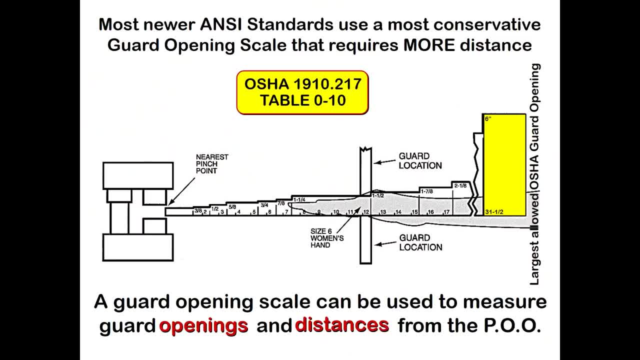 opening that osha recognizes for guards. it's right here a six inch opening, 31 and a half inches away for those of you with a plastic wood. whatever guard opening scales, you notice that last segment usually does not show up because it would make it such an awkward size. i think there's a few that do but remember that. 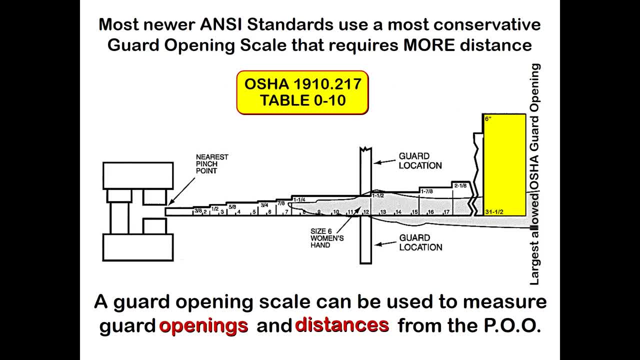 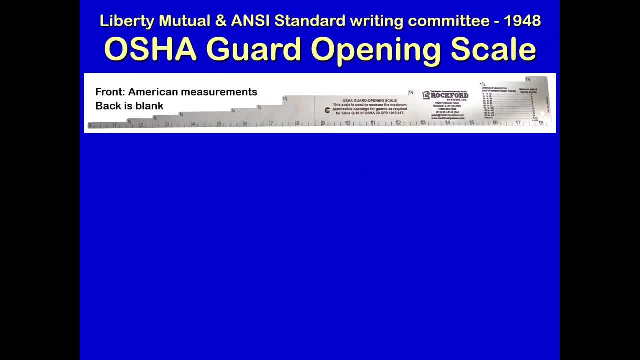 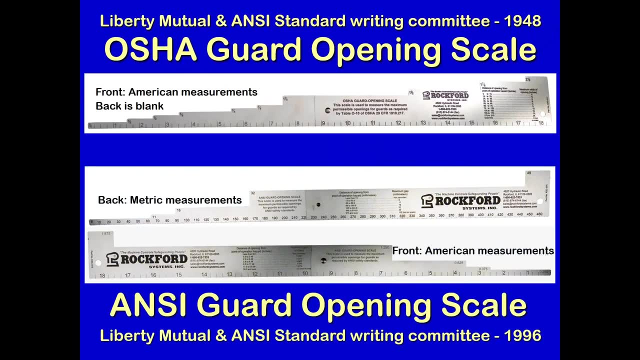 is your largest osha acceptable opening for a size six glove? um, that came from a 1948 study with liberty mutual insurance and the ansi standard writing committee for i think was antip 11-1, which produced a measurement scale that you can use like that and that's what osha uses- state or federal osha around the country uses. 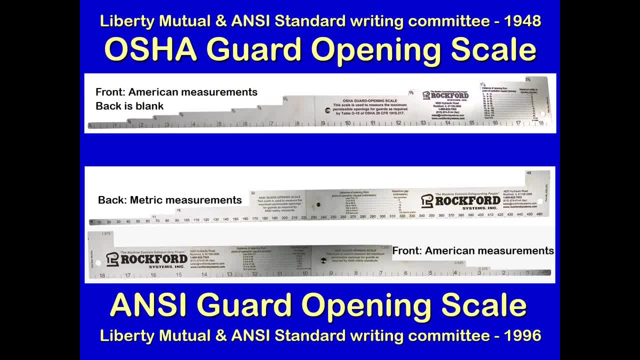 that scale only, which came out in 1948, long before ocean right there. then in 1996, the same two groups got together and made a revised scale based on a woman's size four glove with average finger length. oddly enough, that was because of a study they did that showed there was more asian. 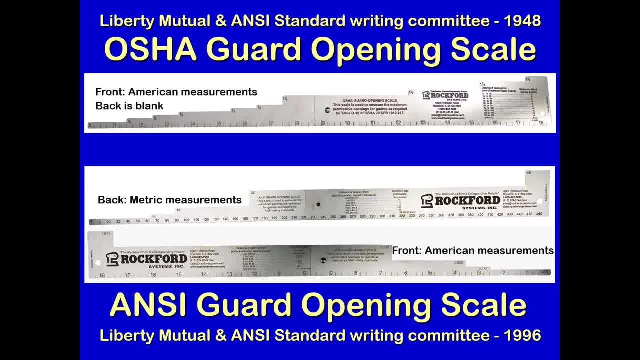 women in the workplace that had very small hands. so that came out in 1996 and, as oftentimes, you first referred to as the ansi guard opening scale, because it's more conservative, based on a smaller hand size. oddly enough, the robot standard talked about the 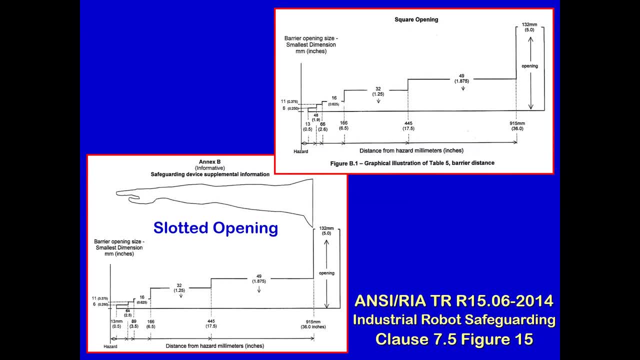 technical report that came out 2014 talks about square and slotted openings in these two drawings and is a match, for neither one of those two guard opening scales based on an isostatic came out of europe, but i think it's an in-between hand size. 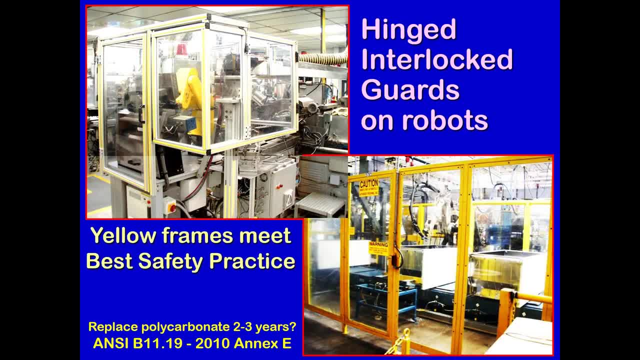 as far as the yellow framework on guarding, like, uh, the bottom right one has yellow framework, uh, because it was painted that way. the top left one here has snap in yellow plastic channels. they're going to be aluminum extrusions to make your guard into a yellow framework garden, if you. 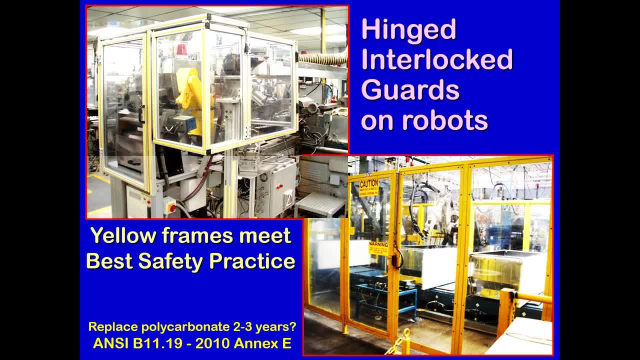 want to do that. that came from an ansi z535 color coding standard as a best practice. it's not an osha issue to have yellow framework on your guarding uh. replacing polycarbonate every two to three years is out there under. well, if you look at ansi b1119, the 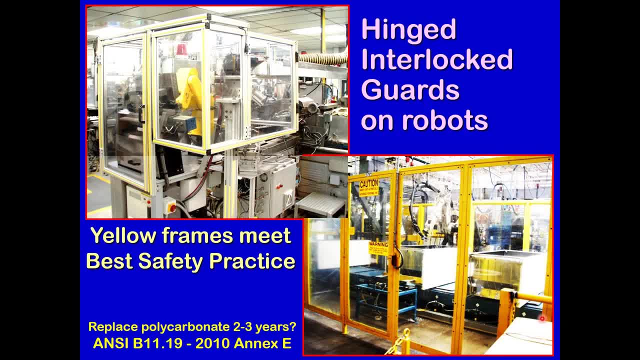 safeguarding method standard from 2010. uh, they suggest doing that, especially if your polycarbonate comes in contact with industrial fluids. cutting fluids and even sunlight will degrade the degraded the impact. protection of polycarbonate over time, especially when you've got somebody standing right now. the 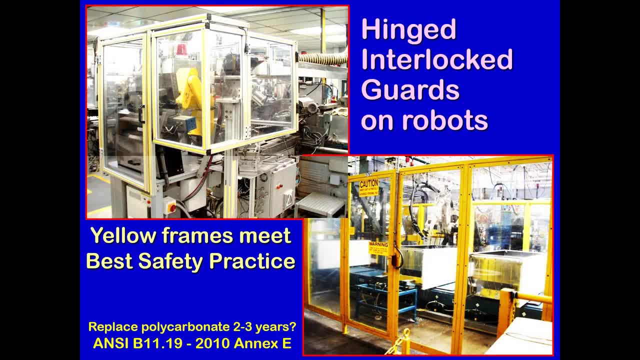 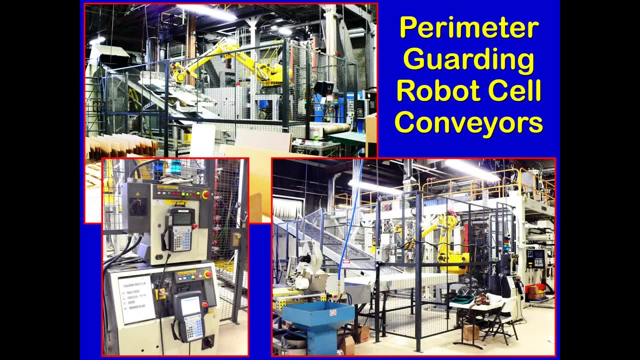 this or in front of this, whatever you want to say, because that's obviously the highest category of protection that you want to provide. when some of these faces behind this perimeter guarding a robot cell with conveyors, well, let's see. all right, see the robot in there. what I'm concerned? 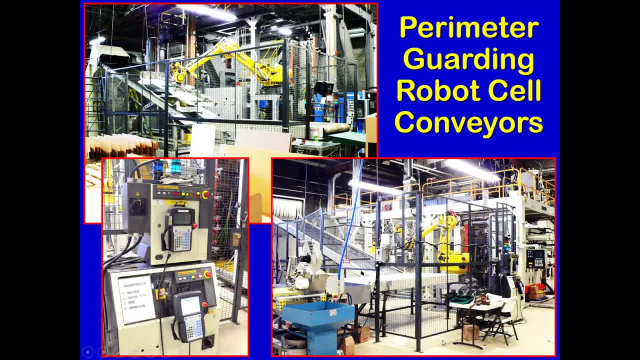 about is down. here there's a bottom right corner. here there's a fence that appears to be maybe 12 inches from the floor, which, according to current standards, is not high enough, low enough. all right, six inches from the floor should be the max, six to seven inches at the bottom, but not 12 inches. 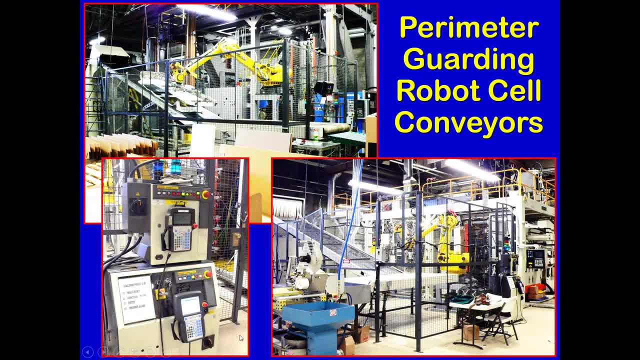 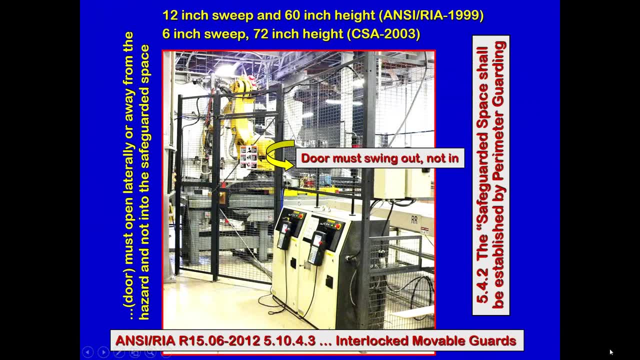 the one that up here. that looks to be within six inches would be my guess, looking at it. so let's see the top line here: a 12-inch sweep. that's the rail at the bottom. the distance from there to the floor was what was prescribed back in 1999. 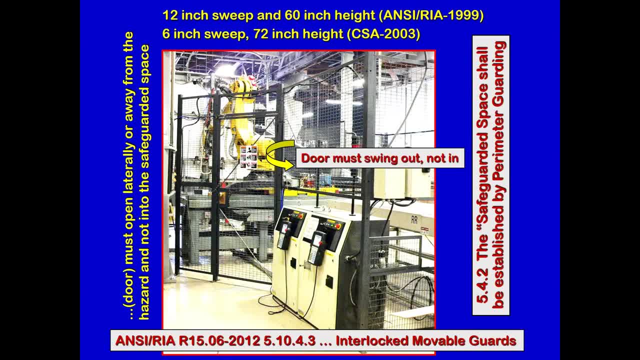 with a 60-inch height. okay, then Canada came along- and Canada usually follows European standards- to say 2003 that you should have no more than six inches at the bottom, which has been backed up by several insurance companies that have been to our seminars and saying, hey, we've had fatalities. 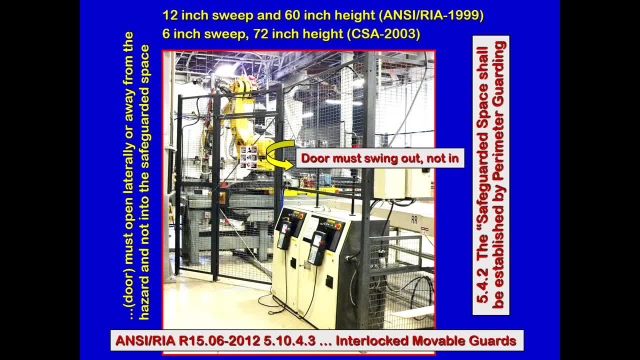 people climbing underneath 12 inches. why? because they start up the robot and automatic everything. everything is set to go and they left their setup sheet on the clipboard inside the safeguarded space. I don't want to call it through doing all this stuff to get in there legitimately, I just sneak under the 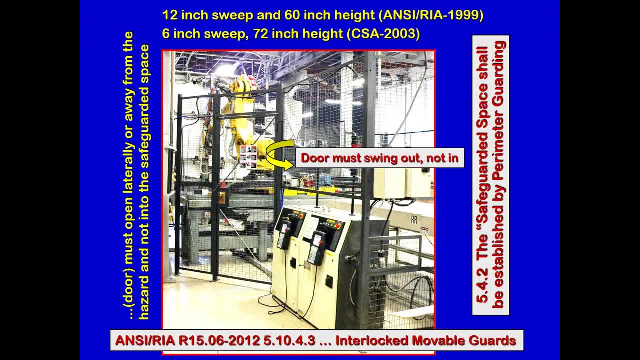 fence because I can see it, it's only a couple feet in here and then the robot comes, you know, pivots around to do unexpected, like if you dress a welding tip or whatever, and you know get some squashes in between the end effector itself. so that's why Canada went to follow the European. 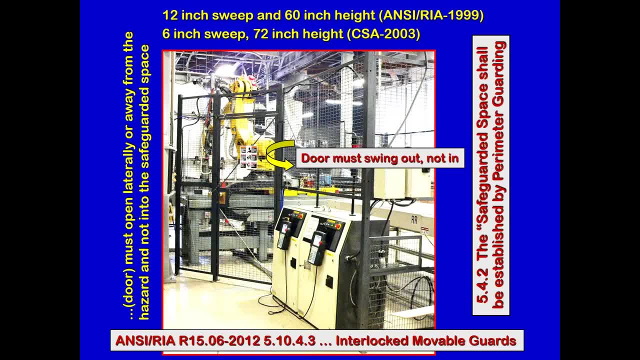 standards with a six inch sweep opening at the bottom and also increase the height. this is from 60 to 72 inches, because robots can maybe, in an emergency stop situation, release apart from the end effector and throw it with a lot of velocity. so making the fence higher is not 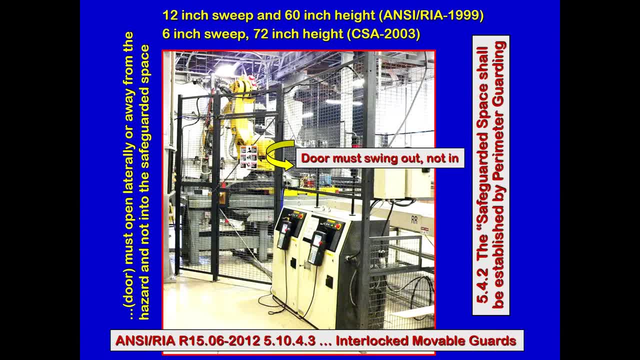 for people crawling over the top, but stuff being thrown from the end effect that doesn't have a retention method to prevent them from doing that. so here's a Canadian standard: six inches at the bottom, 72 inches at the top, and I know, being a custom guard manufacturer, like we, are a lot of. 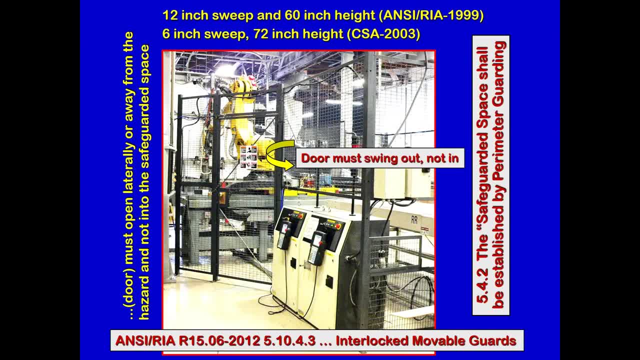 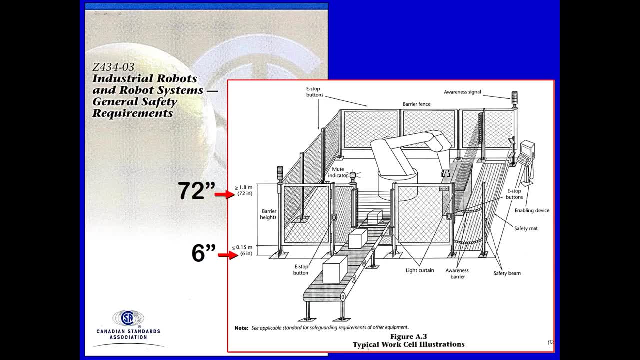 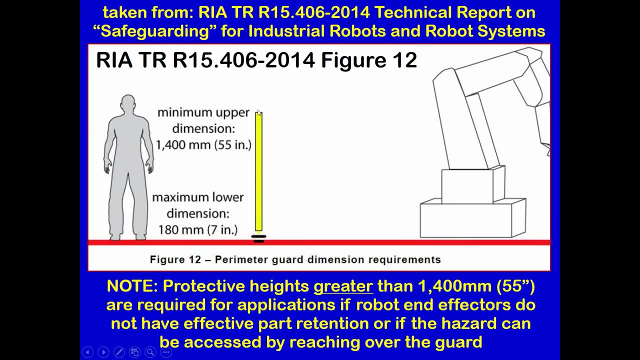 people who want to 84 another foot height on the guard for that very reason. now, if we look at the technical report from 2014, they're specifying seven inches at the bottom and a 55 inch height, with a condition down at the bottom that protective Heights greater than 55 inches are required for. 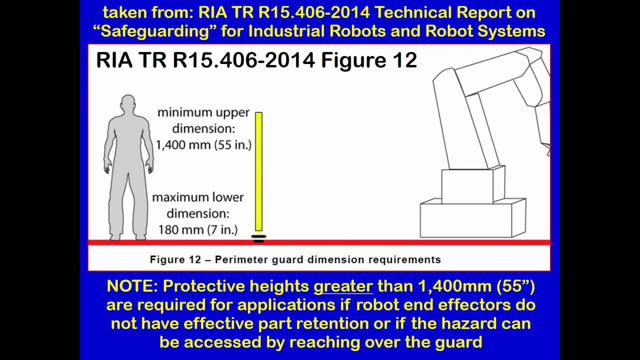 applications, if the robot end effectors don't have effective heart retention or if the hazard can be accessed by over the guard. now, where that came from, I really don't know, because in 1999 you're saying 60 inches. you know Canada and the Europe have gone to 72 and here they're going back to 55. I don't. 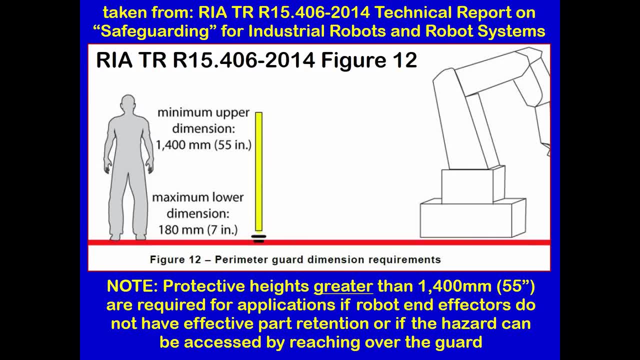 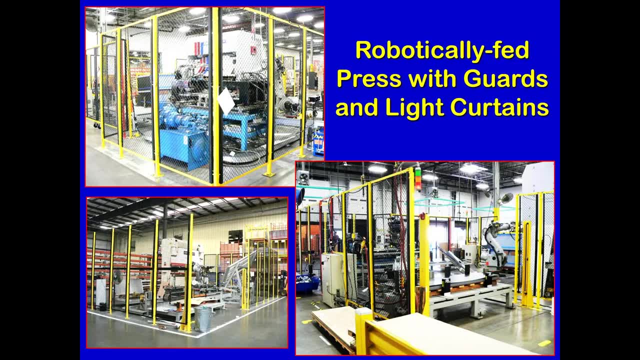 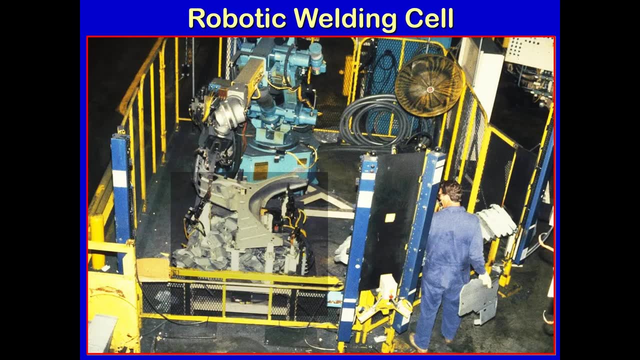 know why that is, but it's. it's in there like that robotically: fat breasts with light curtains, having guards and light curtains around it. okay, you can see some of the fence height issues here. how about this one? this was a local manufacturing plant, at least local to us. that was welding wheel. 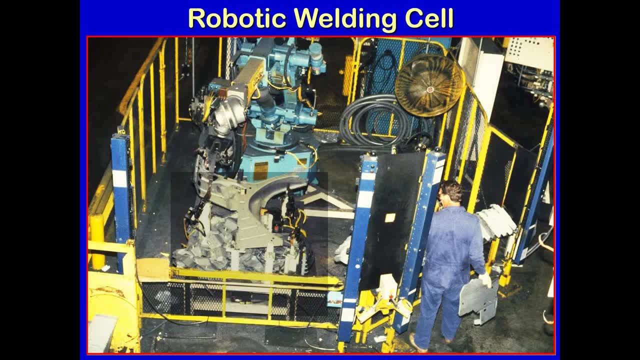 Wells with a robotic cell. first of all, the cell is relatively small in real estate for the size of the robot. um, they claimed that was because of the pull plugs on the arms and elbows, as we've mentioned before. they also had hard stops on the base. I think that has since. 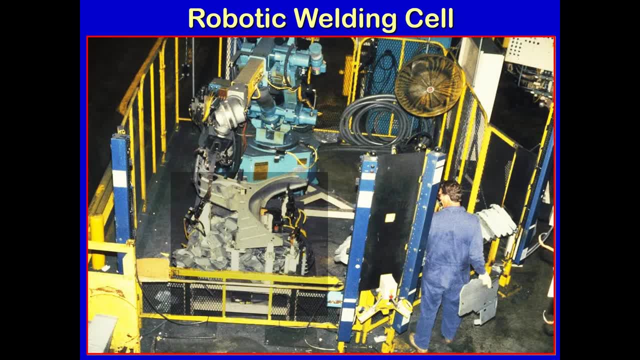 increased as far as the size of the real estate because of the concern that a robot could blow through a hard stop, but at that time that's what was going on. um, this has two light curtains. if you take a look on the right hand side, this light curtain is muted so that operator can load apart. 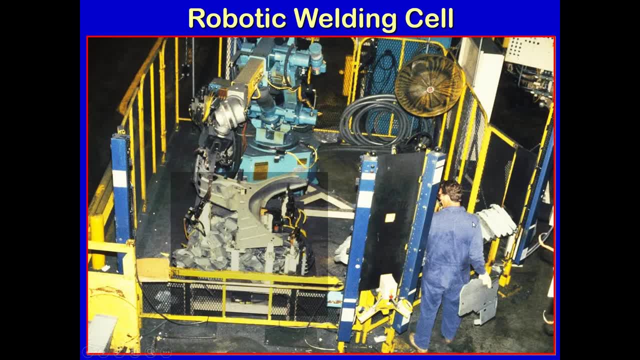 onto a fixture over here, or is? this light curtain is active because the robot is welding the wheel. well, so this is active. when the welding is done, this robot. I'm sorry this light curtain is turned off so the operator can change positions. he can come over, initiate the cycle with the two hand controls and switch. 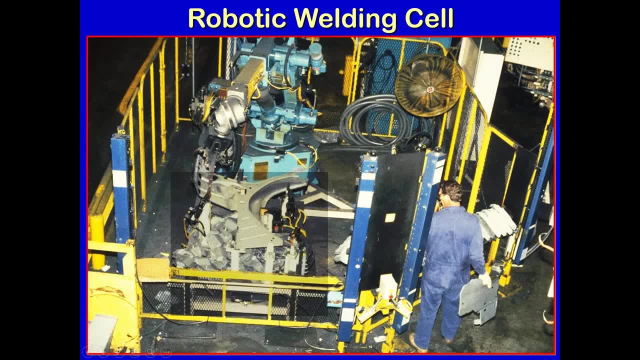 over to the left side. so we've got a fence perimeter, we've got limiting devices of both types, we've got light curtains- two of them- we got a set of two hand controls and we got a partial guard at the bottom, because if you take a close look over here- about 12 inches of the light. 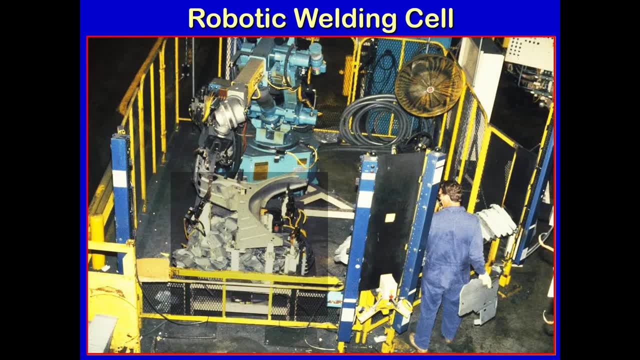 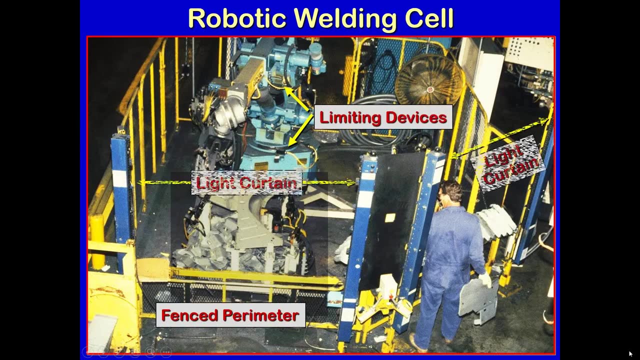 curtain is taped off or blanked out, which would not provide any safeguarding, unless they put the 12 inch high piece of fencing which they did. note that both the interlocks and the emergency stop have a key switch. well, they explained it to me here that when they needed to initiate an emergency, 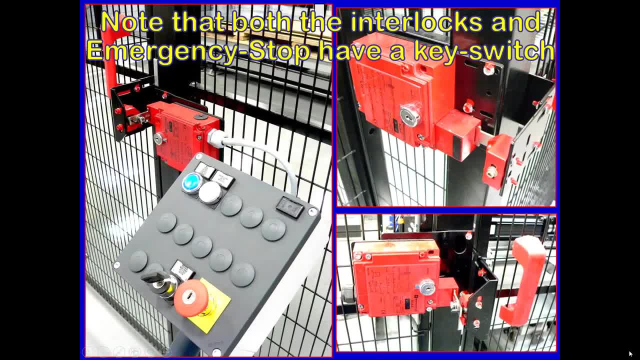 stop through this push button. this latched in the locked position. they could not reset it without a supervisor's key. the supervisor came over, unlocked it and then popped it back to the reset position. allow people to go back to the regular controls to start it up, because what they wanted to do is 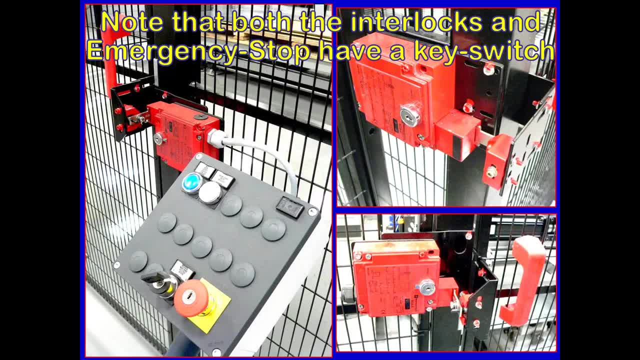 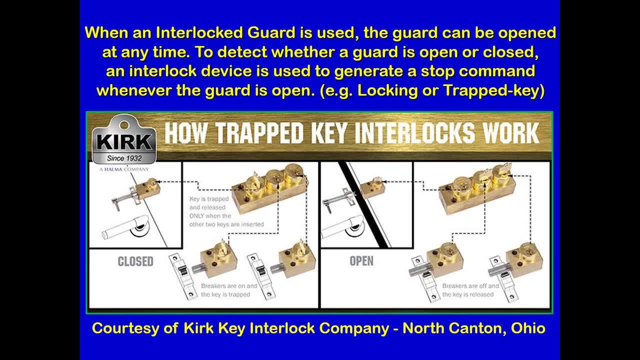 to document what. what caused the emergency stop. we've also got key switches on the interlocks, which could be used in several different ways, one of which is to leave the latch in the extended position so you can't shut the door. you can't shut the door until you have a key to unlock. 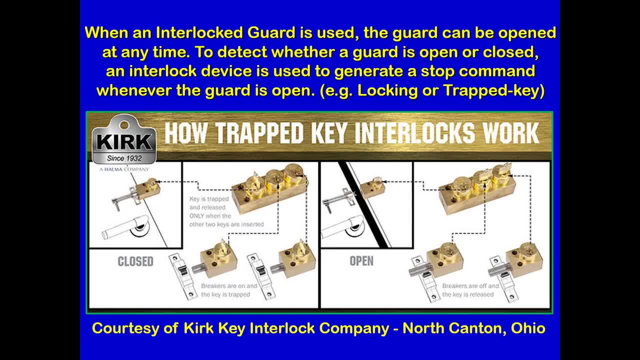 there are other possibilities as well as to why or how they use the key. trapped key interlocks, which is involved swapping of keys at the exchange keys for however many people are involved before you can start up the robot again. trapped key systems. robots sometimes have pneumatic systems. 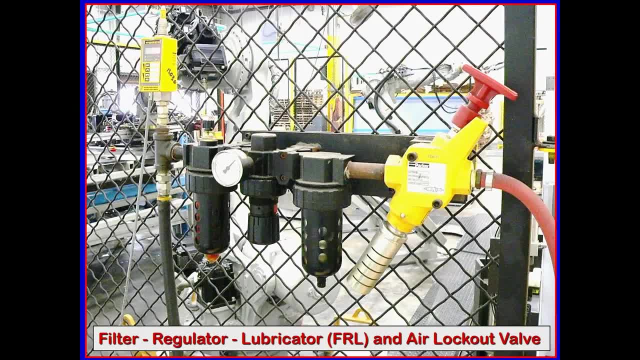 that need to be well. filter out the water contaminants, control the air supply. maybe add lubrication to the airline to minimize the scale of stuff that you get if you run an airline. thrive. so, frls, think up on other machines or something that's using robots along with a three-quarter.